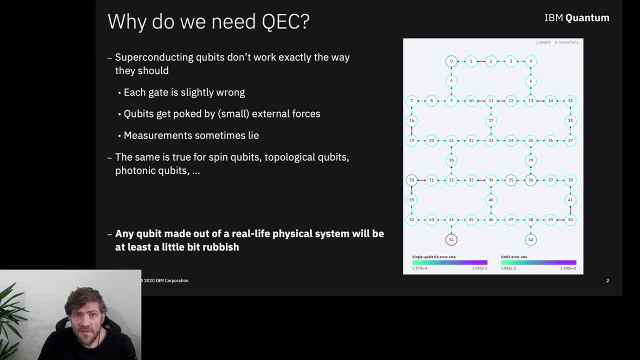 So any implementation of a qubit is going to fall short of the ideal. So a qubit is an abstract concept, the notion of a two-level quantum system that is described by the theory of two-level quantum systems. However, there's always going to be something that's not. 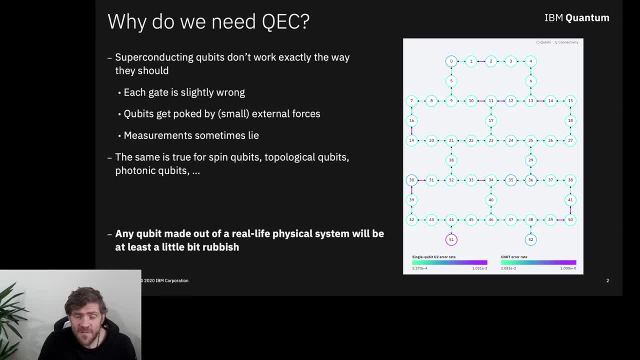 quite right. We make these out of physical systems and they're never quite the perfect two-level ideal that we want. The theory that describes them is never quite as simple as a nice, simple theory of two-level quantum systems that we would like. They're always going to. 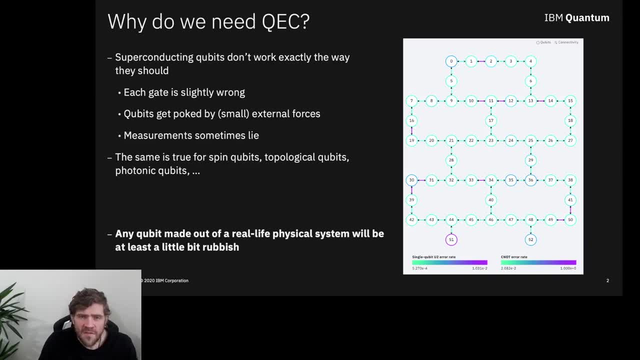 interact with an environment or with a thermal bath, There's always going to be some Hamiltonian inducing interaction. It's always going to be something. Now, in the superconducting qubits that we use in IBM, the two-level quantum system is actually built out of an unharmonic oscillator. 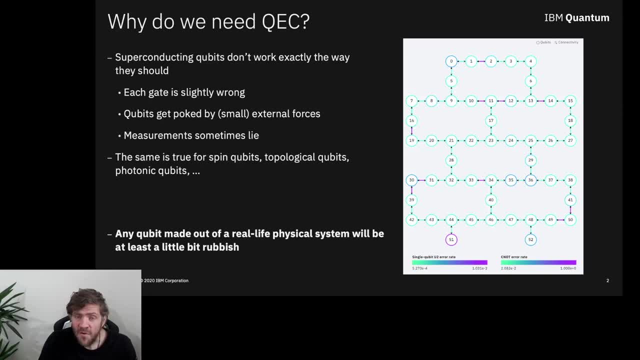 which is not just a two-level system, but is a many-level quantum system. We just isolate two of those particular states in order to use those which are the ground state and the first excited state. So already you can start to see where the approximation begins. 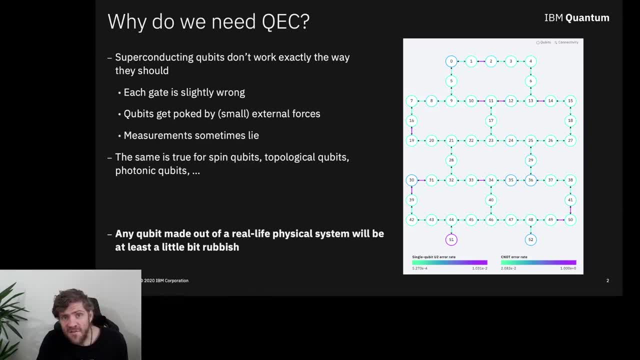 Also the ground state and the first excited state of an unharmonic oscillator are states with different energies. A qubit should not have the notion of there being states with different energies. They are described by an energy-less ideal theory, And so the fact that there are 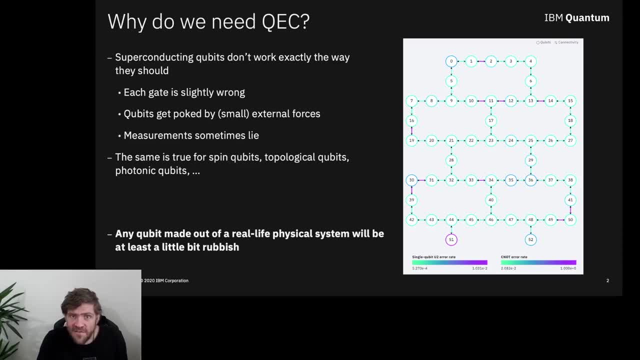 different energies in the qubit means that there are effects that need to be accounted for, one of which being that it's more desirable- if I'm to anthropomorphize a qubit or an unharmonic oscillator- It is more desirable to be down in the ground state, And so we are likely to have transitions where it goes from. 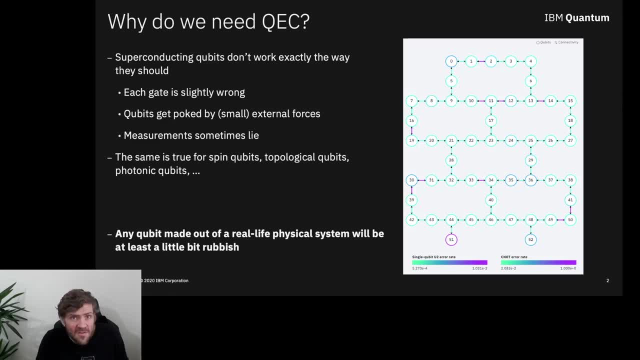 the one state to the zero state, which we shouldn't actually have, at least according to the abstract theory of a qubit. Also, all of the gates that we do are slightly wrong And there are external forces such as radiation or just thermal noise And the measurements. 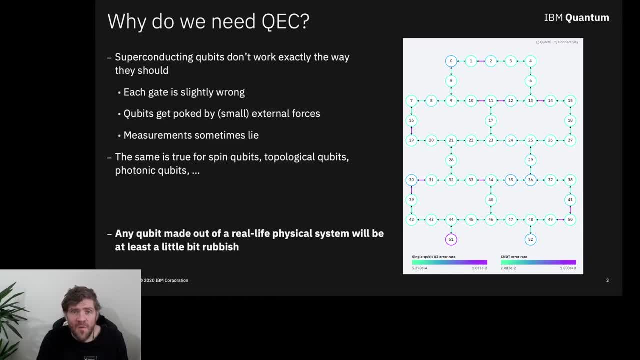 are not perfect. When we do a measurement, we interact with our qubit in a way that we get a squiggly line And some of those squiggly lines are squiggly lines that tell us it's a zero, And some of those squiggly lines are squiggly lines that tell us it's a one. And 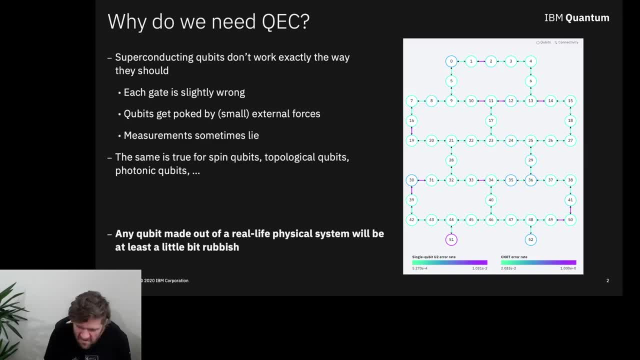 we have to try and work out, given any squiggly line, which is it? Also, there are external forces, So there are interactions with the other qubits on the chip, which means that when we are getting our zero or one from a particular qubit, then we might actually be. 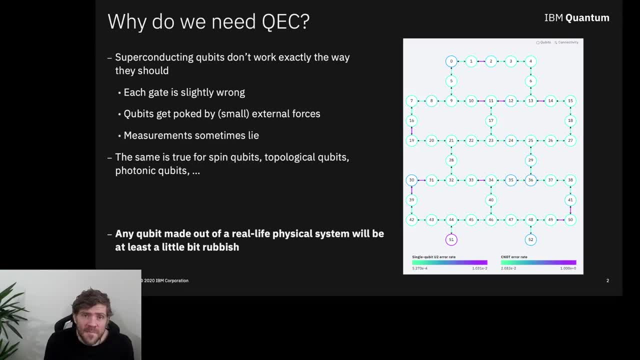 getting little hints about what's going on with the neighbors as well. So there are difficulties in measurement as well that we have to take into account. So any real life physical kit system, whether it be superconducting qubits or spin qubits or topological qubits or something- 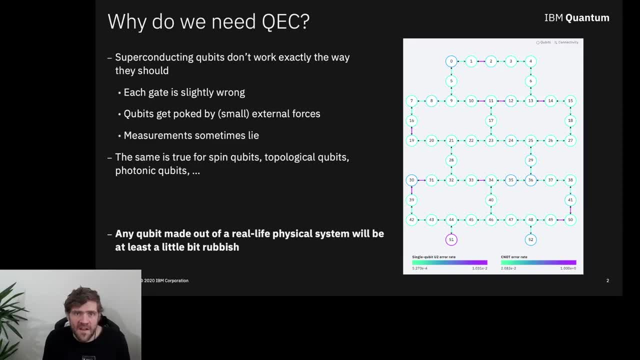 else is going to be a bit rubbish, And so we have to deal with that. We have to take these noisy qubits and try and craft them into the perfect ideal qubit that we always assume when we think about algorithms. And one thing just to note here is that, even though there are many different types of errors, 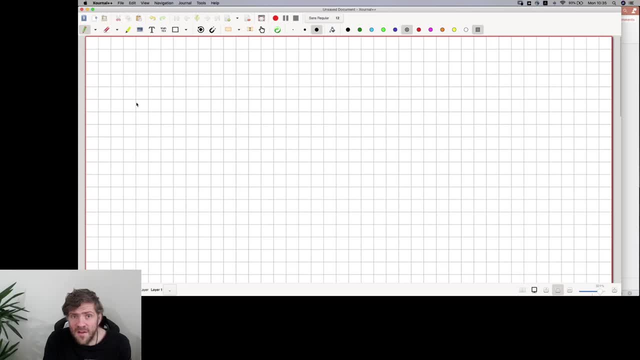 we can actually boil it all down, at least in a simple way, to just three. So imagine that, because of something, Some gremlin that lives in our chip applies some unitary at some point in our circuit. Well, that could be any unitary. So how do we fix any possible unitary that's going to? 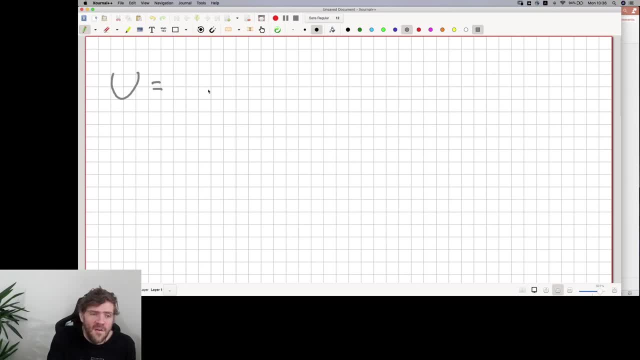 hit any possible point on our circuit. Well, we can use the fact that any matrix can be decomposed into Pauli operators, So we can think of it as some coefficient times- the identity plus some other coefficient Times, the Pauli x, plus some other coefficient times, the Pauli y, alpha, beta, gamma- comes. 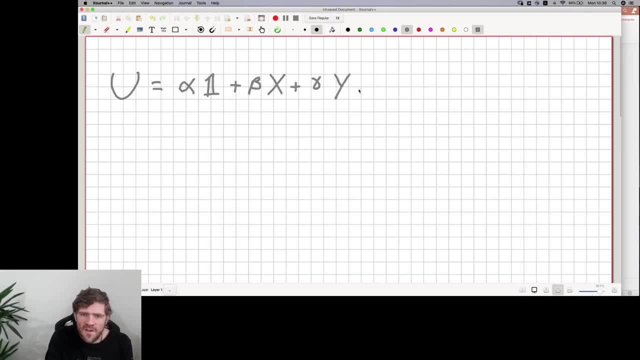 next, I know you all want me to be very exact with my Greek letters, And then some coefficient times, z. So this is a perfectly general way of writing a single qubit unitary. So if we're thinking of a single qubit unitary being applied by some error, 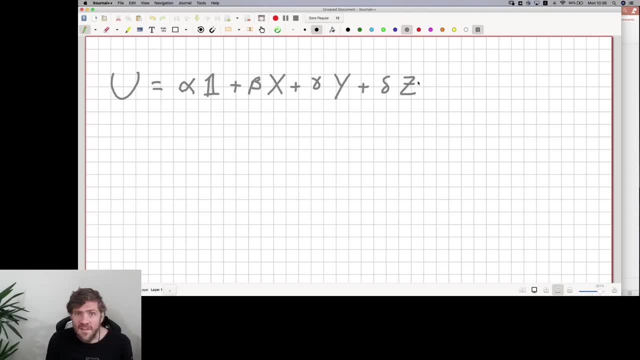 process in error, We can see that this is what we get, And because it's composed of an x, y and a z, when we apply it to some state, then what we get is basically the superposition of our original state, plus what would have happened. 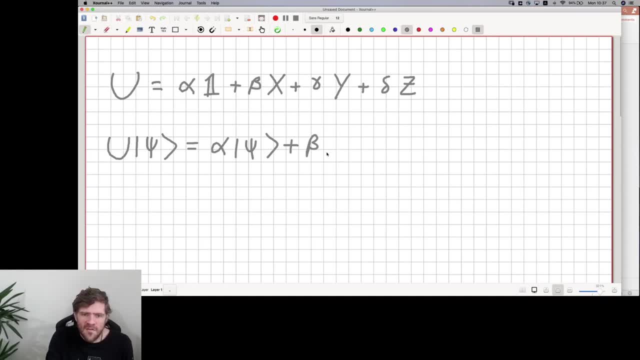 if we had just applied an x to the qubit Plus? what would have happened if we had just applied a y to the qubit plus? what would have happened if we would have applied a z to the qubit? So here, actually, this state psi could be a multi-qubit state, And so I'm glossing over. 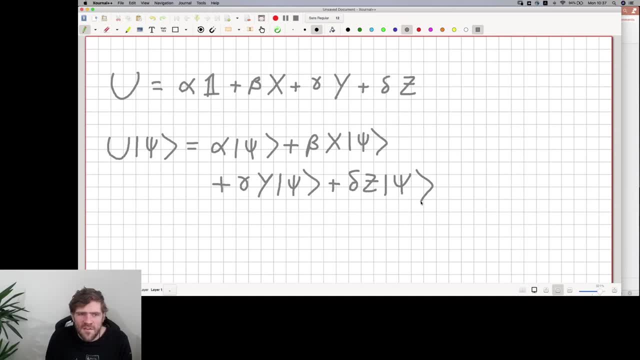 a few little details, But hopefully you get the impression that we can think of any unitary applied in error as being as if we had either done nothing or done an x or done a y or done a z in superposition. So if we can figure out some way of detecting whether we've done an x or a y or a z in error, 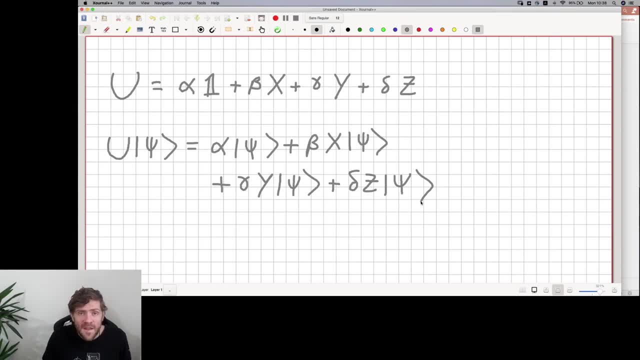 then we can apply it in the case of any unitary, And similarly for two qubit unitaries. we can decompose these into two qubit values, And so it's like a pair of Pauli errors have occurred And so, basically, we can make everything just into: have we done an x error, a y error or 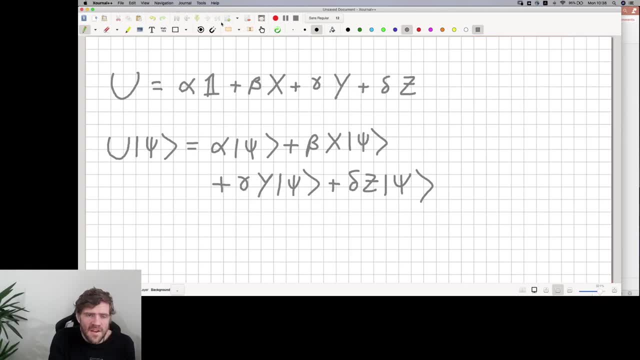 a z error. And in fact we can even make it a little bit more simple than that, because the y Pauli is proportional to x times z. So we could just put x times z in where we put y before, and it would still work. 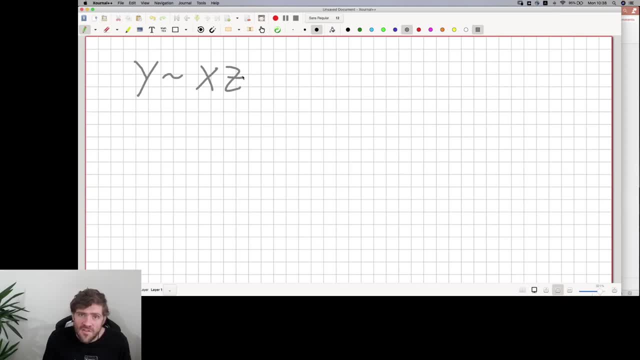 So now it's whether we've got just an x or just a z, or x and z together is what we have to detect. So it's sufficient just to be able to detect x's and y's, And that's it, Thank you. 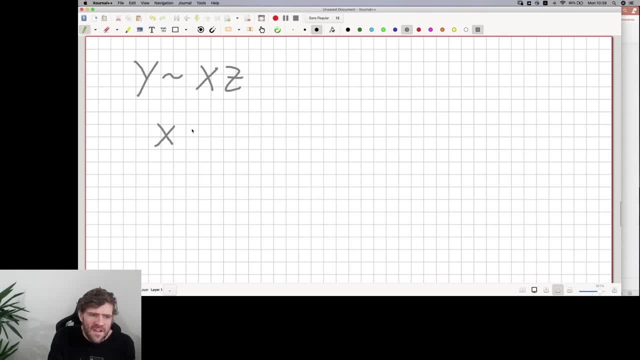 We then simplify the problem into two phases. And so there you have it, an X. This just takes one to the zero, and then it takes an М to one. And so what is an X? Well, often we will refer to this as a Bitflip error, at least when it is applied in error. 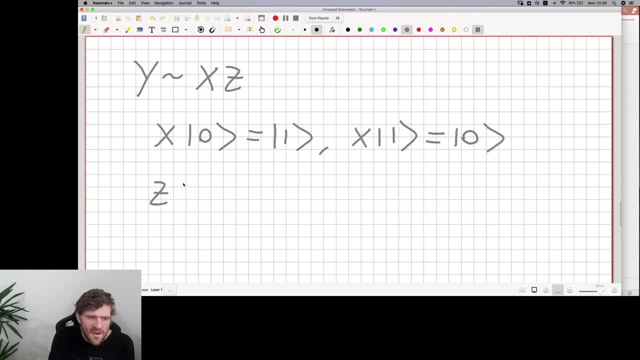 because it is the operation that takes one to zero and zero to one. Of course, I've just said them in the opposite order than I've written them down, but nevertheless plus to minus and minus to plus. so because of that we call it a phase flip error, because of: 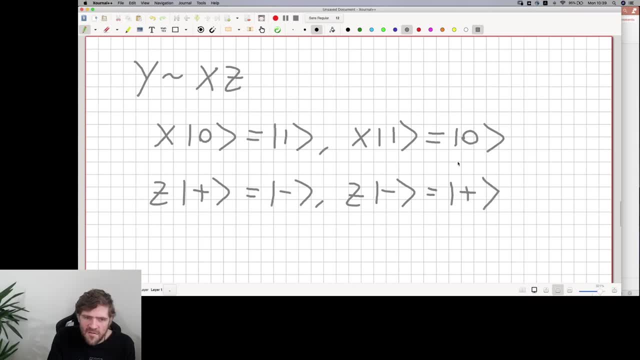 course these differ by the phase in the middle of the superposition. So if we just have the ability to detect both bit flip errors and phase flip errors, then we have the ability to detect everything. Now there's details, there's weird things that can come up and you can write a. 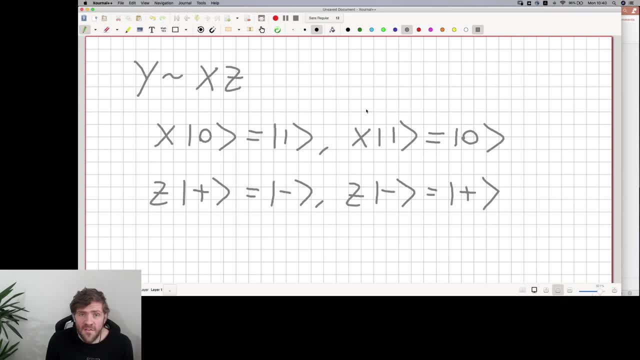 whole paper about. but that's basically what you need. If you can detect x and z, then any spurious effect by any unitary or any other operation can be decomposed into the Pauli's and therefore decomposed into just having some superposition of bit flips and phase flips. and by detecting 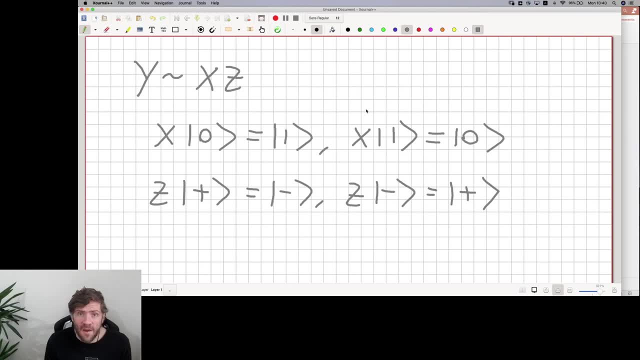 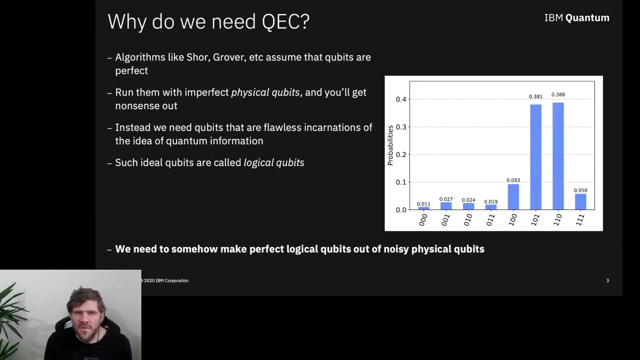 bit flips and phase flips and being able to correct them, then you can correct basically everything. So how Are we going to detect bit flips and phase flips? Well, let's head back to the PowerPoint. So why do we need quantum error correction When we have algorithms like Shor and Grover? 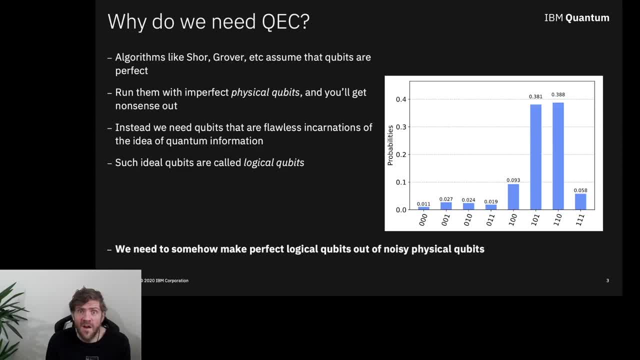 and so on. we assume perfect qubits, We assume this ideal abstract form of a qubit and if we use actual, physical qubits to run the algorithms, then the imperfections in those algorithms are going to build up over the course of the algorithm and mean that at the end everything's a bit rubbish. 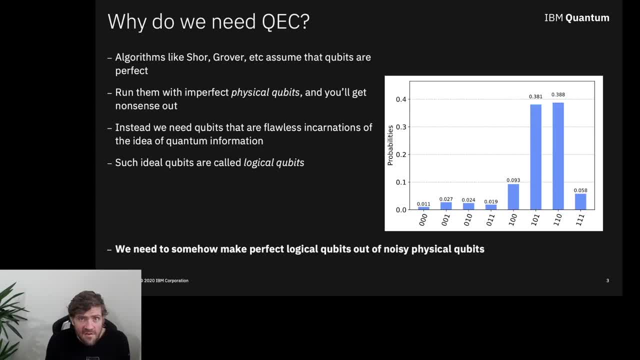 So here is a histogram from an example of Grover's search algorithm, where it is searching for two particular strings rather than one, and you see that there are two strings that have very high probability, but we would expect that these both have probability of 50% that 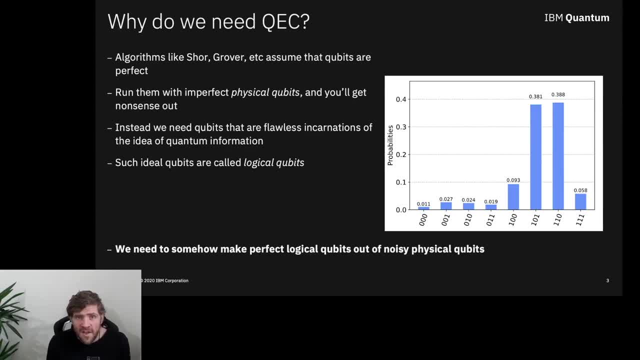 when we read out the final output, we are going to get, with 50% probability, one of these correct answers or the other one, But in fact they are only more like a third rather than a half, and there is quite significant probability for other answers as well. Those should all be zero, but they're not zero, and 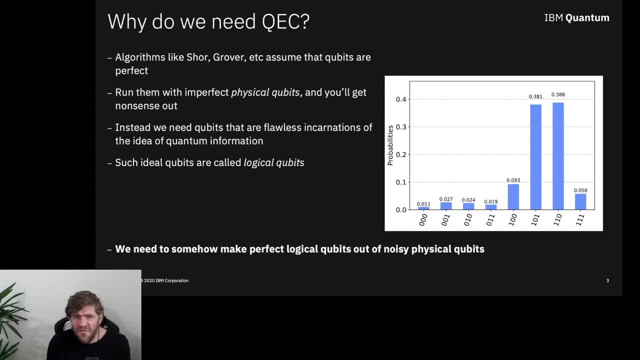 that's purely due to the effects of noise. and this is only a three qubit example of Grover's algorithm, which is a pretty trivial example. It's only searching through eight different possibilities, which you can do using methods other than quantum computing. Thank you. 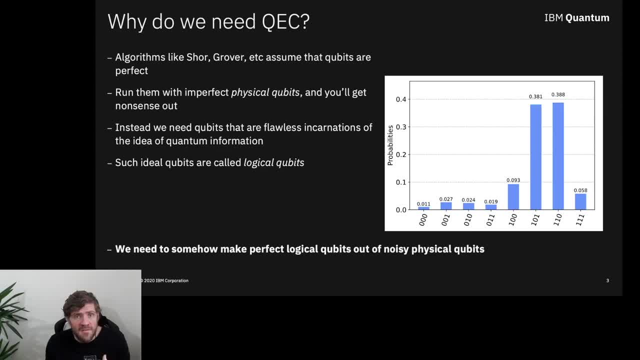 Quite simply So. when we scale this up to useful examples of a search algorithm, then these spurious results get higher and higher, the correct ones get lower and lower, and there's basically no point to running them. So we need to sort out these errors somehow. 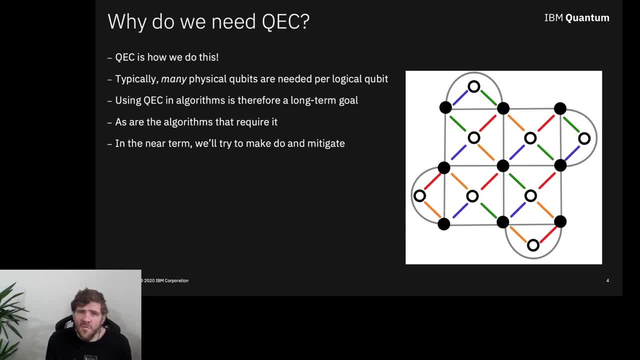 And we do it by quantum error correction. So one of the important points to note in quantum error correction is that we need many physical qubits to make one logical qubit. A physical qubit is the kind of thing that you use at the moment in IBM Quantum Systems — the 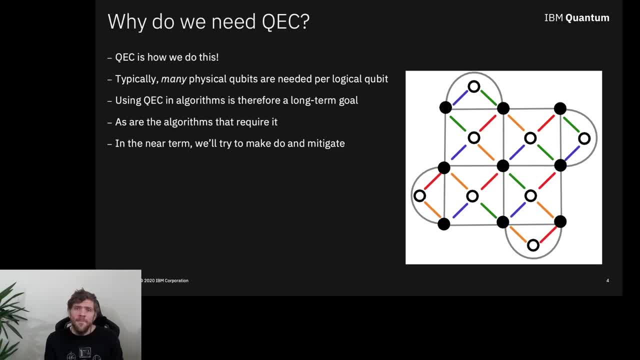 actual things on the devices, the things that are noisy. Logical qubits are the things that you assume that you have when using an algorithm — something perfect — something that suits the ideal of what a qubit should be. The way we build a logical qubit is by adding the defined irresistibility, so that we get 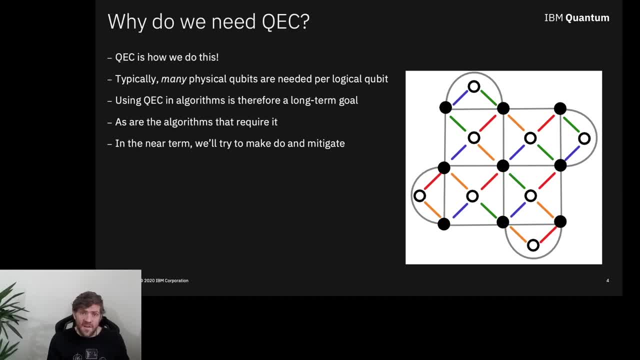 is by taking many physical qubits and combining them. So the diagram that you see on the screen at the moment represents a D equals three, surface code. It has 17 qubits, so nine of them depicted as black dots and the rest depicted as these white dots, and it requires many controlled operations to 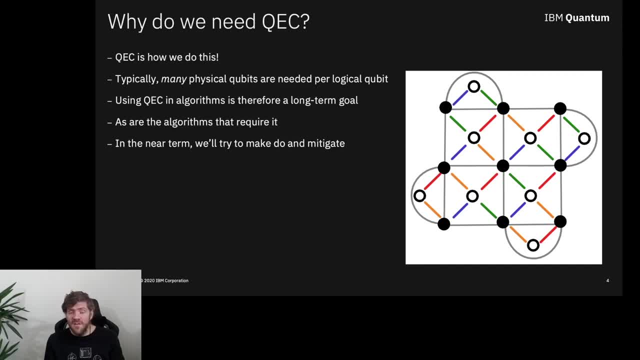 be performed. so all of the colored lines represent controlled operations that we need to be performing each syndrome measurement round and we need to be repeating these syndrome measurement rounds constantly. We'll talk about what a syndrome measurement round is later, but this is just to impress upon you how. 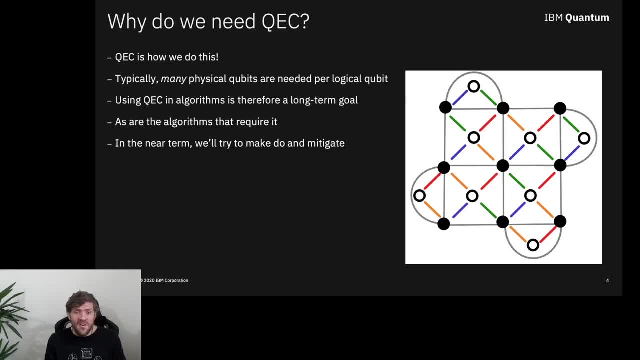 difficult it is to build a logical qubit. You need lots of qubits and you need lots of gates to be performed, and this is just a minimal example. This is just like stage one of showing that you can build something that reduces the errors. a. little bit. It's not even what you need to reduce the errors significantly, or enough to do quantum error equation, and we haven't even got on to the idea of how we actually do computations on these qubits. So yeah, you need to combine a lot. 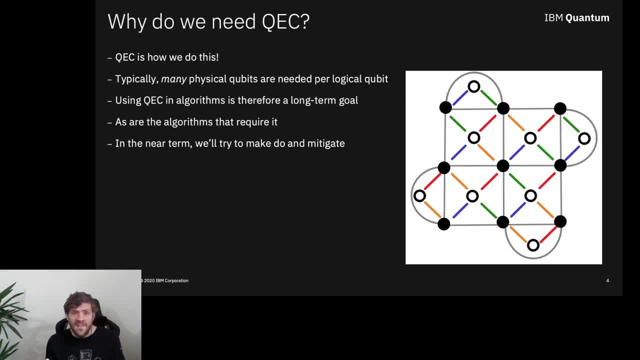 of resources to get fault tolerance- and we'll talk more about that In the near term- we don't use the full force of quantum error correction. So quantum error correction is this great theory which proves that we can do scalable and fault tolerant quantum computing if we 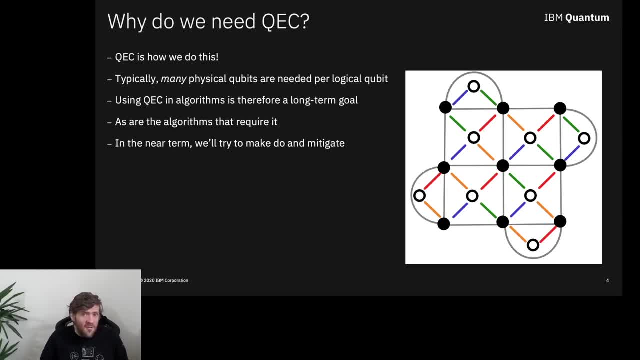 have enough qubits but it requires so many qubits as overheads is something that we can't really get started with at the moment. In the nearer term, there are more quick and dirty methods that we can use to clean things up And really we can kind of expect to see a continuous transition between error mitigation. 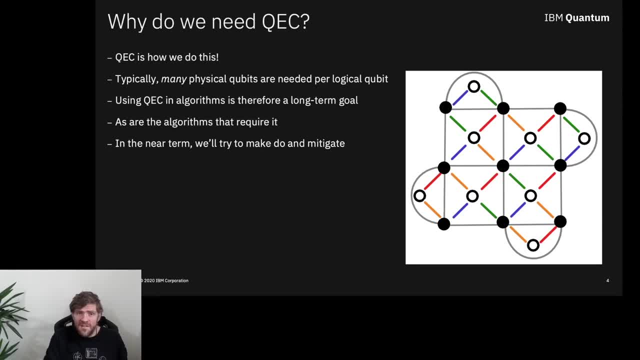 and error correction, where we start going from quick and dirty and navigate towards clean and perfect, theoretical but huge overheads. And yeah, so that's quantum error mitigation, quantum error correction and the journey to between them, which is something that we'll be doing over the next couple of weeks. Thank you very much. 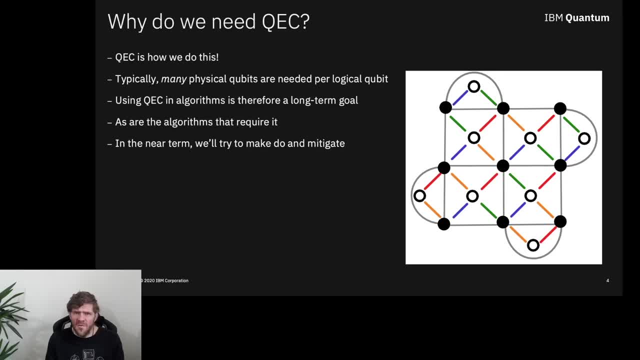 Decade or so, but we won't talk too much about mitigation in this lecture. Okay, so, as I hinted at earlier, we're going to be looking at the ideas behind error correction, starting off classically and then going to quantumly, and we're going to look 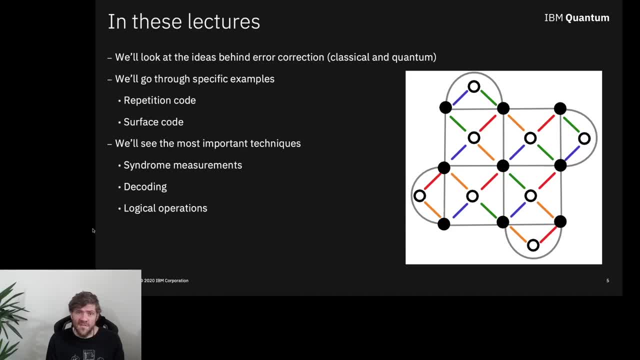 through specific examples of the repetition code and the surface code, and we're going to kind of see how the surface code can be thought of as a generalization of the repetition code. Now we'll also look at some of the most important techniques behind everything, both in the context. 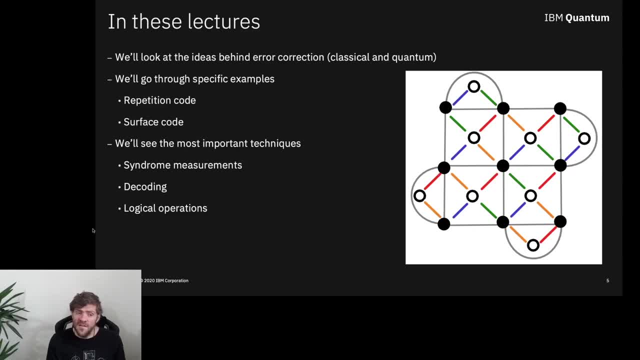 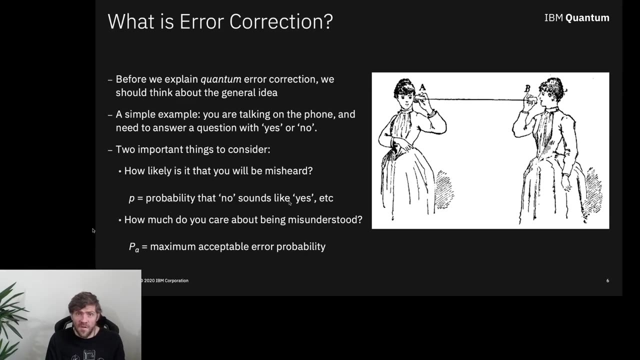 of the repetition code and the surface code, which are doing syndrome measurements and performing decoding and doing gates on our encoded information, which is very important if we want to actually use it in a computation. So let's begin with what is error correction in general? So error correction is a very simple example of this. You can think you're just talking on the phone and you just have to answer yes or no. 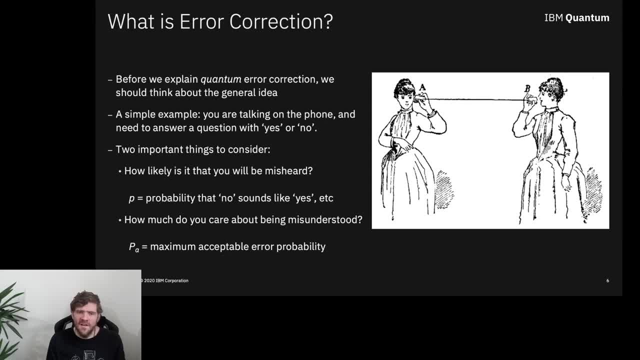 So that is a bit of information that you are sending. There are two pieces of information that you, two probabilities that you should be taking into account when doing this. One is the probability that you will be misheard. So it's quite a weird error model. I'm going to propose to you now where there's some probability that a yes sounds like a no or a no sounds like a yes. 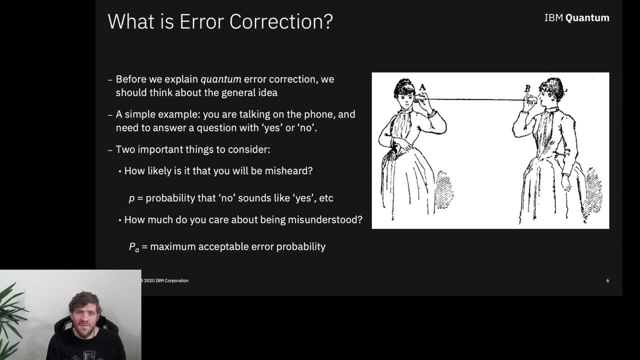 Just take that strange error model, because it makes things simpler for us, Of course. really, when you're talking on the phone and there are errors, it's more likely that your yes sounds like a or your no sounds like a, rather than them sounding like each other. 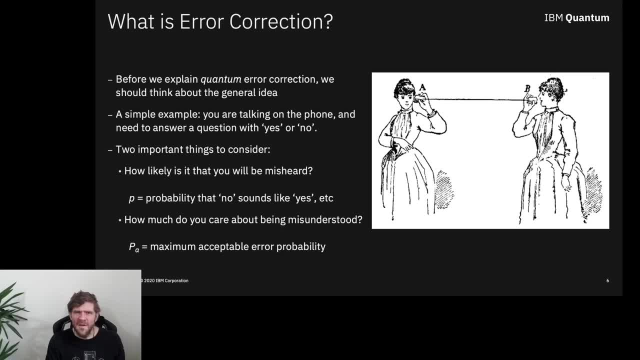 Well, I suppose that white noise that I tried to make there is maybe a bit old fashioned. digitally Now you might be more likely to get it. or just silence. Maybe there's some machine learning Running in the background trying to think about what you were answering and deconstruct, and reconstruct it from the noise. 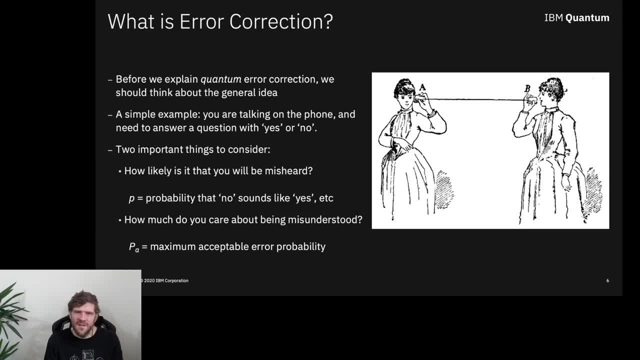 So maybe that would turn yeses to noes and noes to yeses. Anyway, let's move on. So there's a probability that you get misunderstood and there's also a probability that you should take into account which is the maximum acceptable error probability. 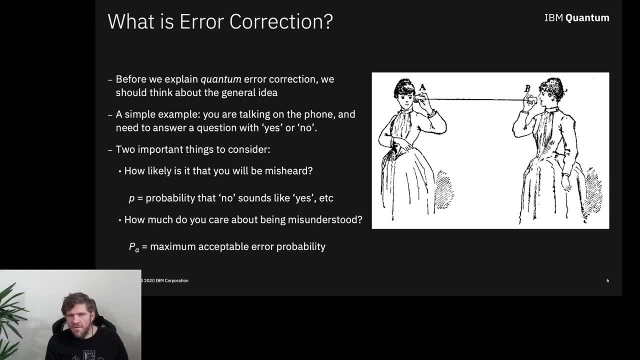 So if you are just saying yeah, yeah, no, no, no, You don't even not even listening to the conversation, If you don't care, if you're misunderstood, if you are the, the, the person in charge of a nation state, and you're being asked matters of life and death, then probably you care a bit more. 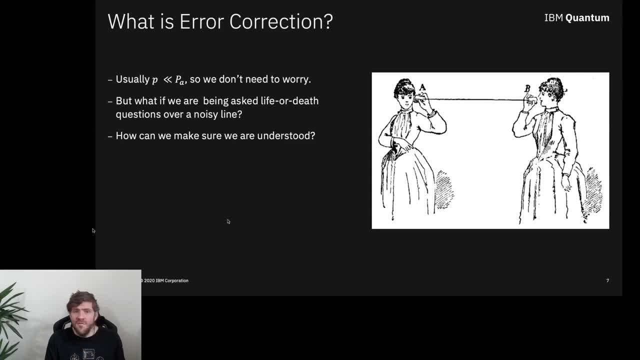 Hopefully you do So. usually in our everyday lives, the probability of there being an error is very much less than the probability of the threshold probability that we care about. So that's that. OK, So we don't need to worry. But what if we do need to worry? 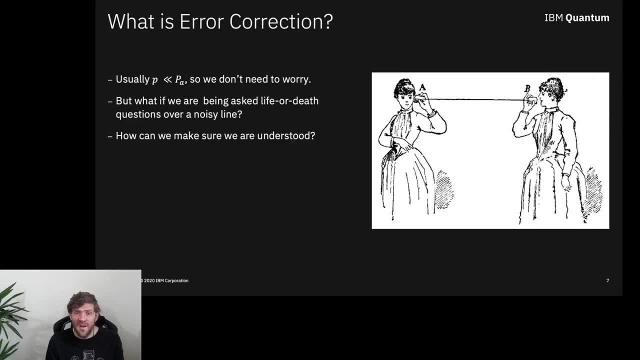 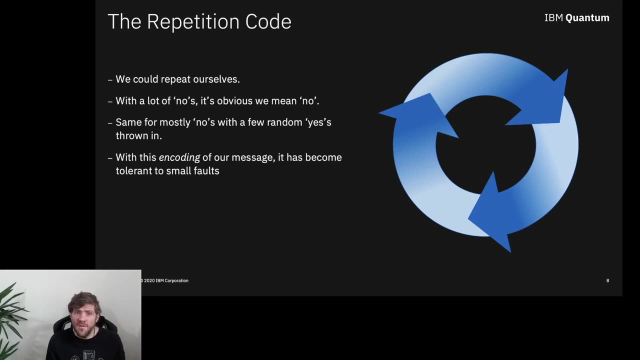 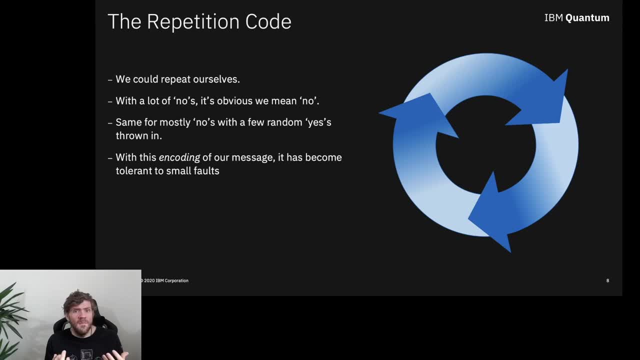 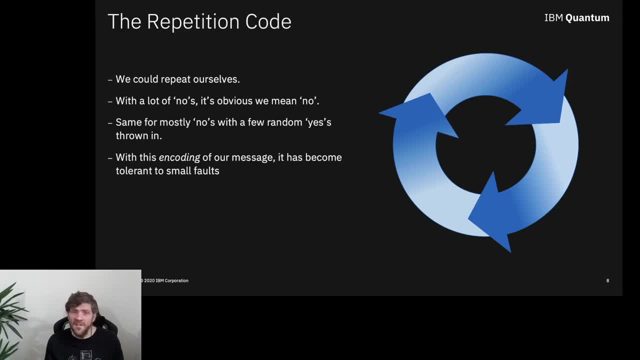 Now that sounds pretty negative to me. If I heard someone say that, I would think that probably means no, rather than hear the yeses and think: well, they just overruled everything. So we have taken our message, which is just a simple bit- a yes or a no- and we have transformed it to a more complicated message, a bigger message, one that is stored on more bits, which is just to repeat it. 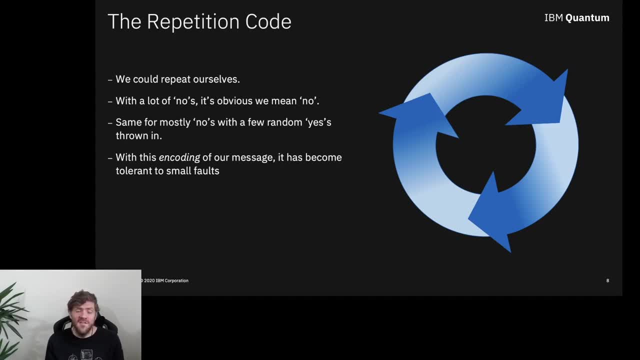 And then we have also decoded our message by looking at the majority to see whether it sounds more like a no or more like a yes. So I've already mentioned the decoding there. But we can also think: what is the probability that a misunderstanding will happen? 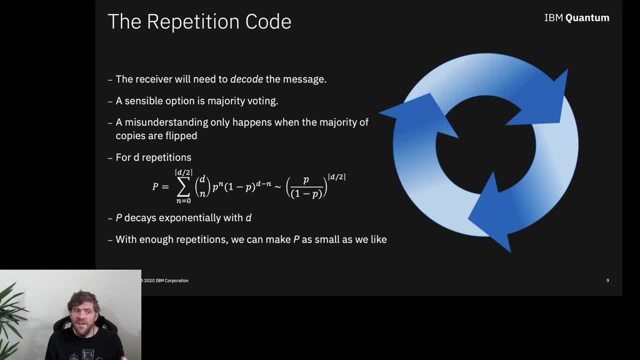 And a misunderstanding will happen only when the majority of the copies are flipped. So if we only say it once, then the probability that the majority of the copies are flipped is just the probability that that one is flipped. If we say it twice, then we get to a point of ambiguity. 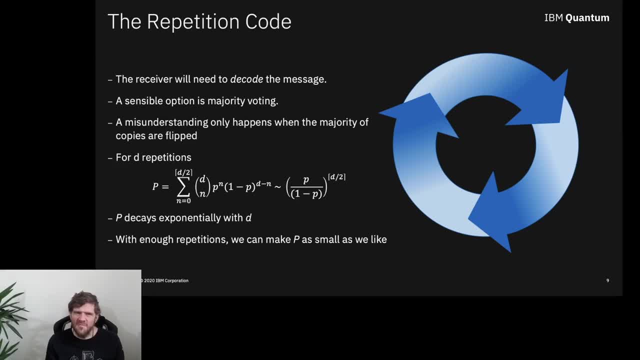 If one of them is flipped then we can see that something went wrong, but we're not quite sure how to correct it. If we say it three times, then it has to get flipped twice. Two of them have to be flipped to go from a majority yes to a majority no or vice versa. 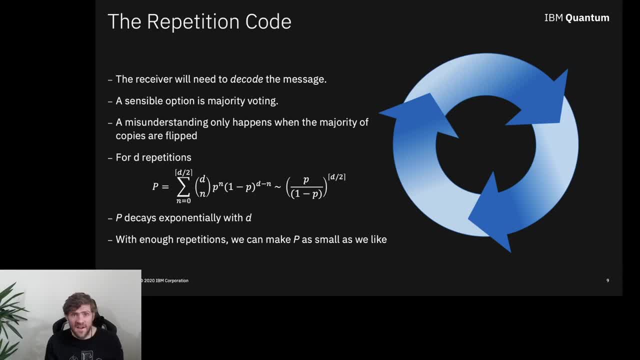 So the probability there goes quadratically with the probability of a flip on a single bit. For d repetitions we can come up with this big sum with a binomial coefficient: The probability that each bit will flip, The probability that the rest of the bits will not flip. 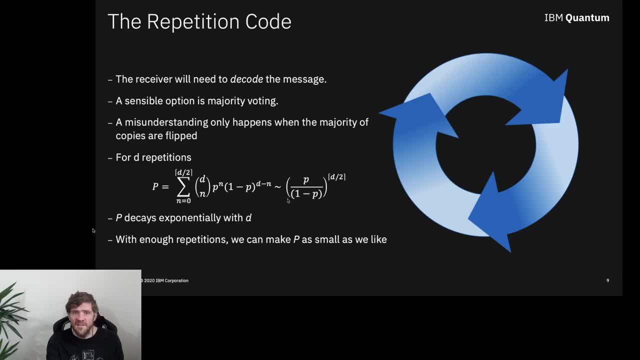 And what we find is, at least in the case that there is low probability, that it kind of scales as the probability divided by one minus the probability, all to the power of the number of repetitions divided by two. And yeah, that's basically what we get. 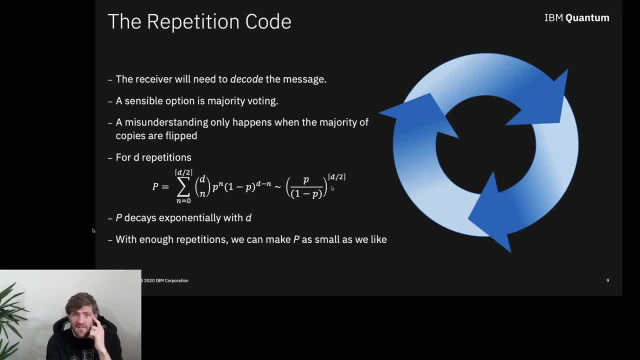 This ceiling function is because we want to remove the ambiguous case where it's 50-50.. Now here we've got rid of the binomial coefficient by just saying, okay, our p has to be sufficiently low. That binomial coefficient is actually quite important in other quantum error correction codes. 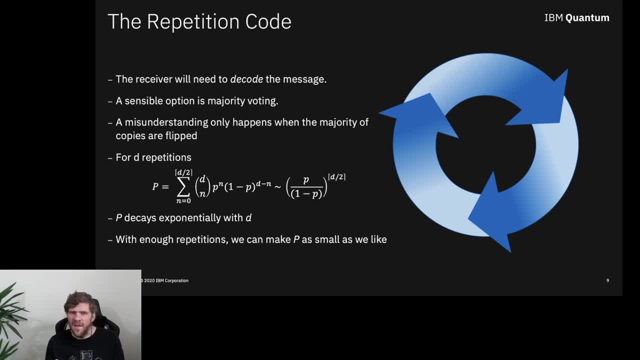 because it tells you: well, how low does your p have to be for this to work? For the repetition code, which is very simple, the probability of a flip basically has to be less than half, to mean that you're more likely in the state you should be in than the other one, and you're fine. 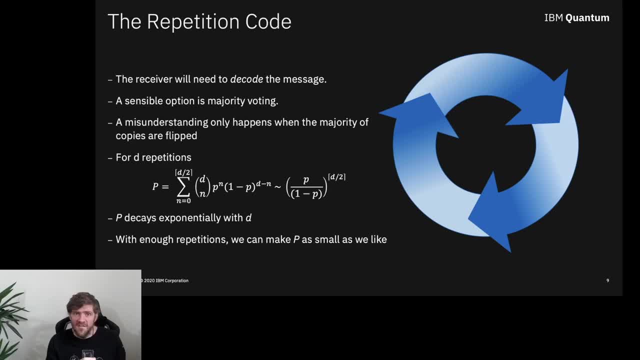 For other error correcting codes, the binomial coefficient is going to have a more effective effect and will mean that you have to be lower than another threshold. So for the surface code you have to be lower than 1% errors, as they're typically quoted. 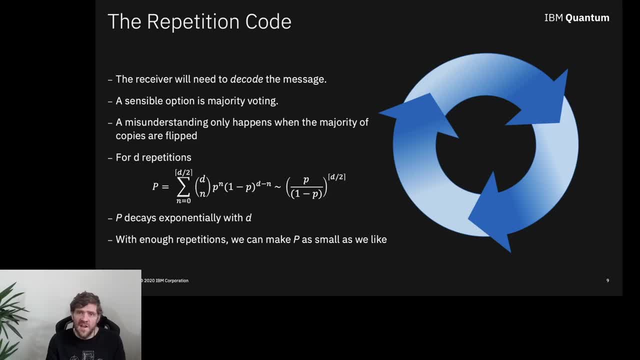 So that's a good figure in order for you to have this kind of scaling. But yeah, in general you will expect that the probability will decay exponentially with d, which is your code distance. In the case of the repetition code, that is the number of times you repeat. 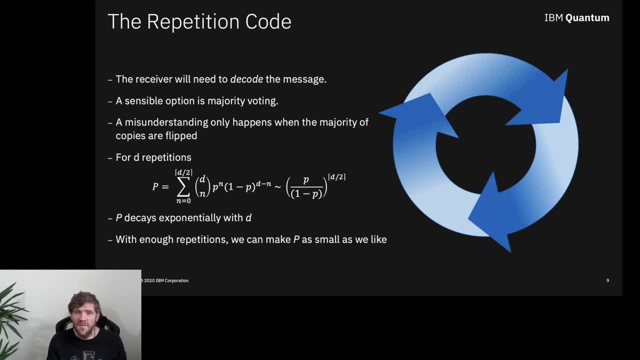 In the case of other codes it typically varies somehow polynomially. For the surface code, the code distance is the square root of the total number of qubits you use. But yeah, you would typically want that your probability of the errors overwhelming your encoding and causing you to decode incorrectly. 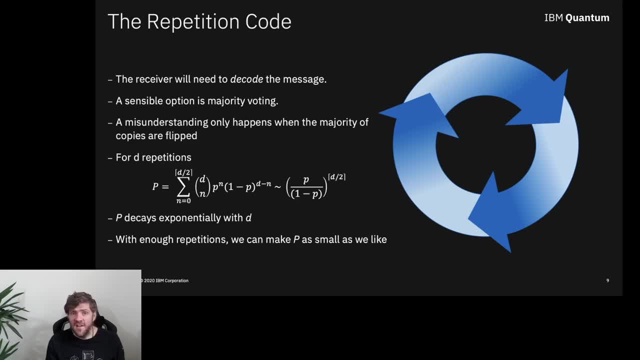 should be exponentially decreasing, with some parameter d which scales somehow as a power law with the number of bits or qubits that you use. Yes, and then in that case you can just use a big enough code and you can make the probability that it all goes wrong. 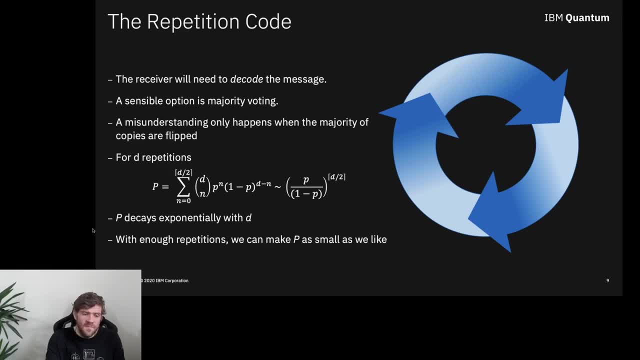 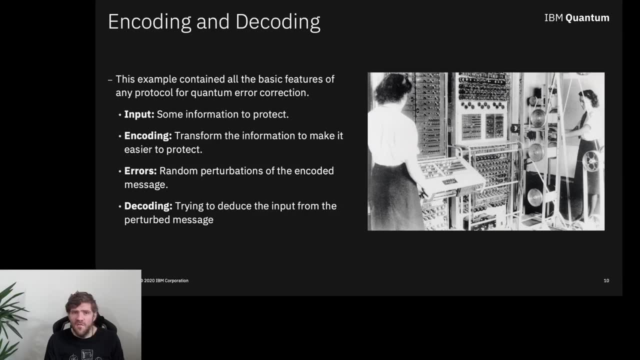 as small as you like, Right? So in this example we had all of the basic elements of any protocol for error creation or quantum error creation, which is: you have an input which is some information to protect. You have an encoding which is some way to transform that information. 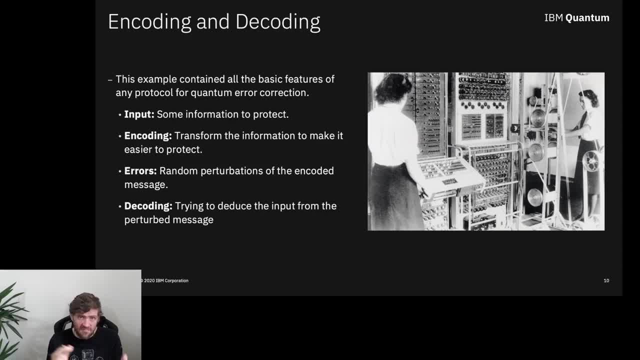 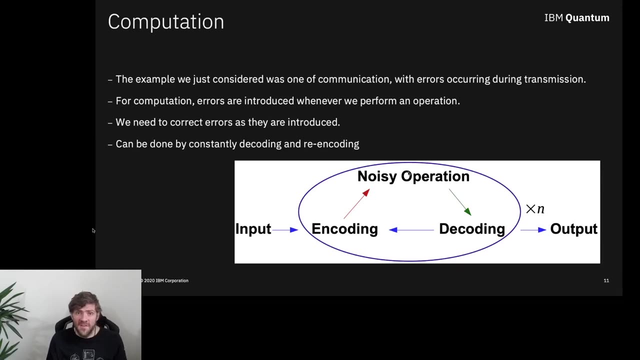 to make it easier to protect. You have errors, which are some weird random things that happen, And then you have decoding, which is you try to deduce the input from the perturbed message. So this example was really one of communication. 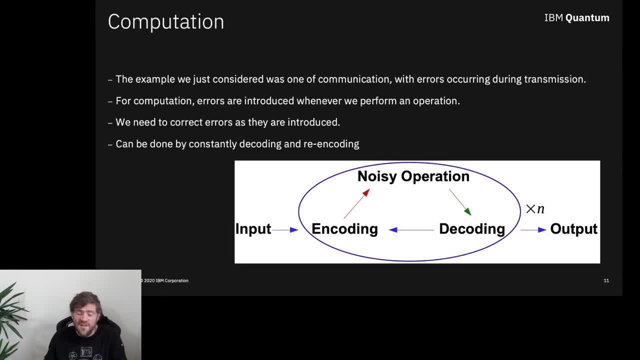 where you have an input, you send, and the sending process is what induces the errors. And then you receive, and then you decode, and then you get the error, the message sorry, and you go on with your life For computation. 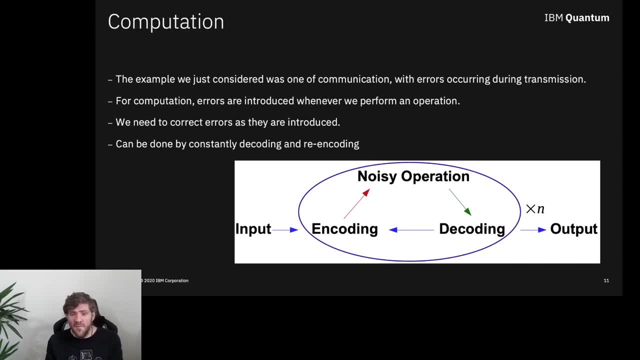 it's more of a dynamic process where errors are introduced whenever we perform an operation, And often the way we perform an operation depends on there not being an error. So if there is an error, we have to change our strategy for performing the operation. 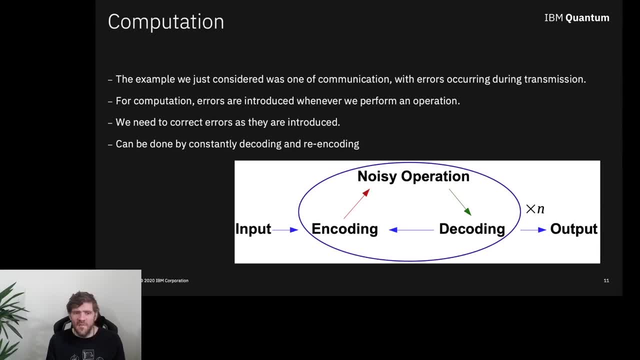 to mitigate for that error. So for that we need to catch errors as they are introduced, to detect them and to mitigate for them in some way, or even, ideally, just to correct them. So that can be done by constantly decoding and re-encoding. 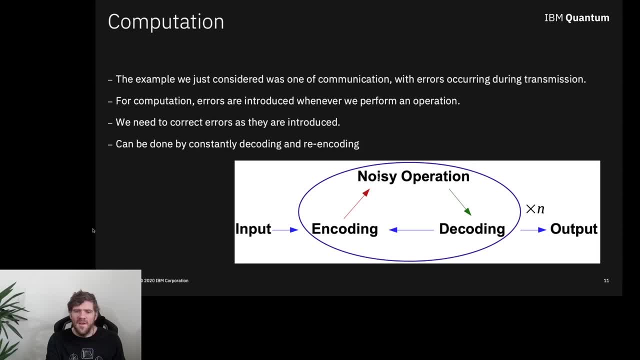 So we can have an input, we encode it and it goes through a noisy operation. it gets decoded and then it gets re-encoded- noisy operation, blah, blah, blah, blah, blah, blah, blah, many, many times, as many times as it requires. 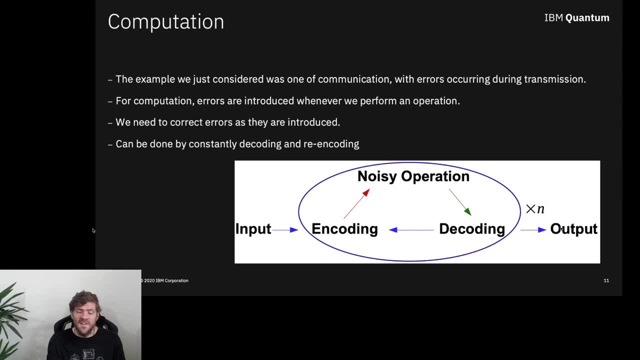 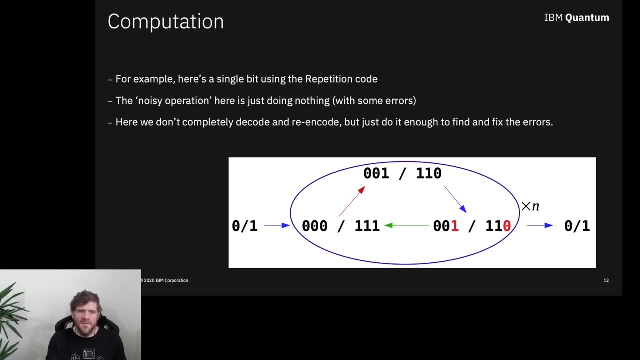 to keep it safe throughout our computation, and then at the end we get an output. So, for example, we can do that with a single bit in the repetition code. Here the noisy operation is just doing nothing, except that that's going to be. 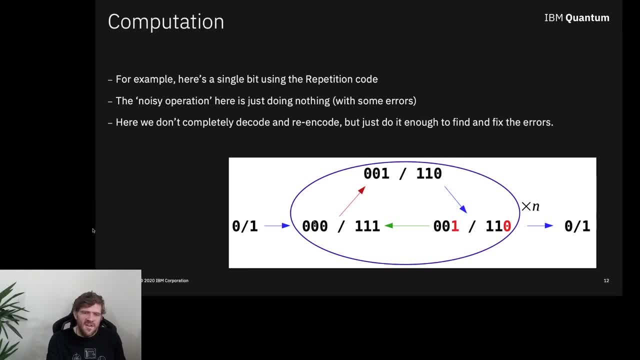 that's going to have some errors occur in general, And from this we can see that actually we don't need to completely decode and re-encode each time, but just enough to fix the errors, which is going to be very important for the quantum case. 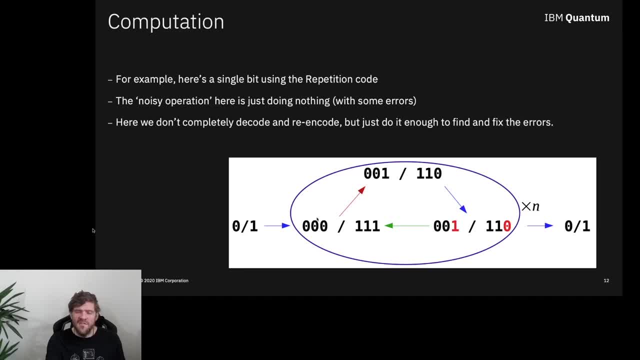 So we take our input, which is either a 0 or a 1.. If it's a 0, we turn it into 000.. If it's a 1, we turn it into 111.. And then this goes through a process where 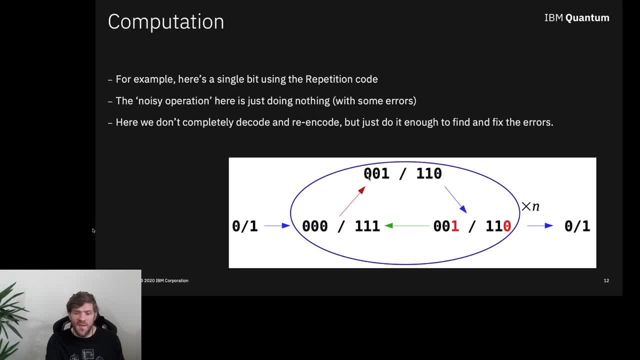 in this case the bit on the right is flipped, So we get 001 if we had an original 0,, or 110 if we had an original 1.. And then in our decoding we just see that that's obviously the odd one out. 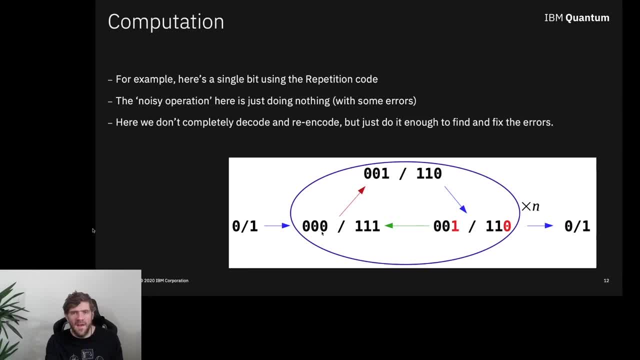 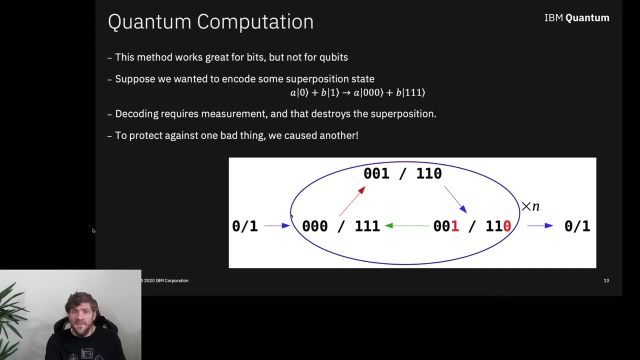 so that's where the error happened, and then we flip that back and so on and so forth. We just keep on detecting and correcting, correcting any errors that occur, and then at the end we get an output. So this is a method that works great for bits. 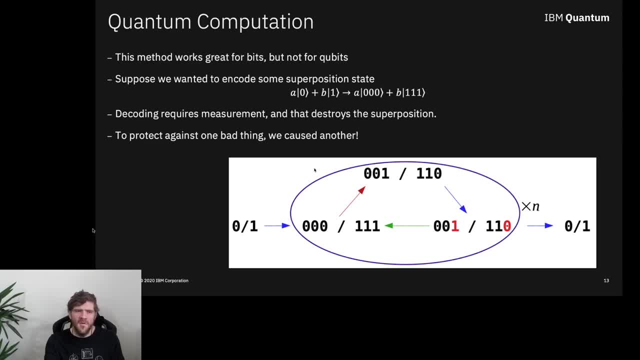 but not so much for qubits, because suppose we wanted to encode a superposition state, so some superposition a0 plus b1. Then the 0 would transform to 000, the 1 would transform to 111, so we'd get this superposition. 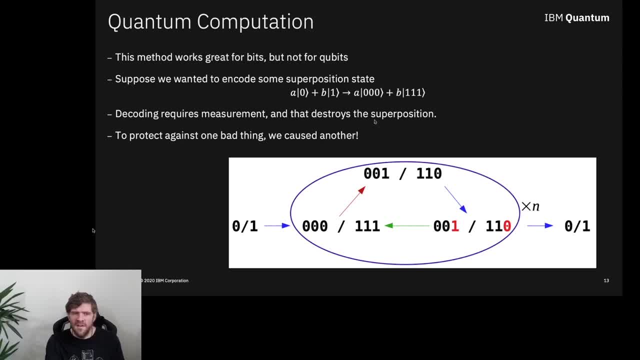 which is an entangled state of 000 and 111.. Now the decoding requires measurement and there has to be measurement because we have to extract information about the system in order to get information about what errors have occurred to it. We need to get out the information. 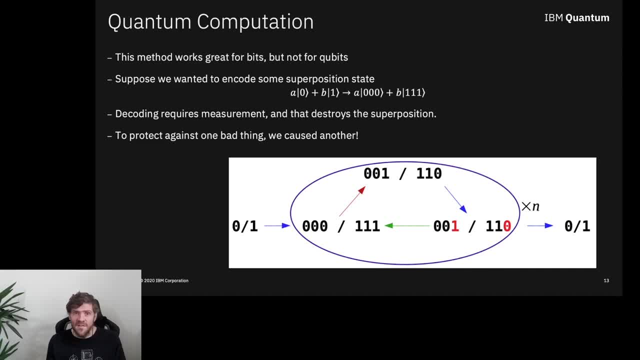 about what errors have occurred. The only way to get out information is to perform some sort of measurement, And if we just measure the 0s and 1s, that destroys the superposition. So we have allowed ourselves to correct bit flips by performing the measurement. 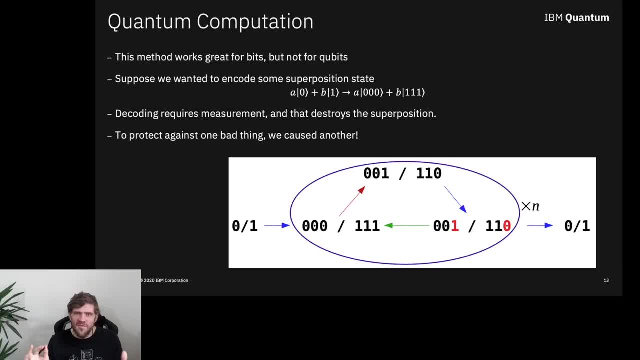 but we've caused essentially something worse than a phase flip, which is to destroy the superposition. So, to protect against one bad thing, we caused another, but that's obviously not what we want. To solve this, we need to be more careful. 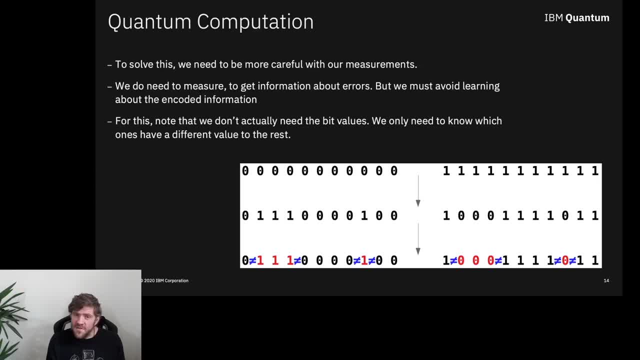 with the way we do the measurements. We do need to make measurements, but we should only extract the information we need to extract, which is some clues as to whether or not the errors have occurred or not. So what we need to measure is not the qubits or the bits themselves. 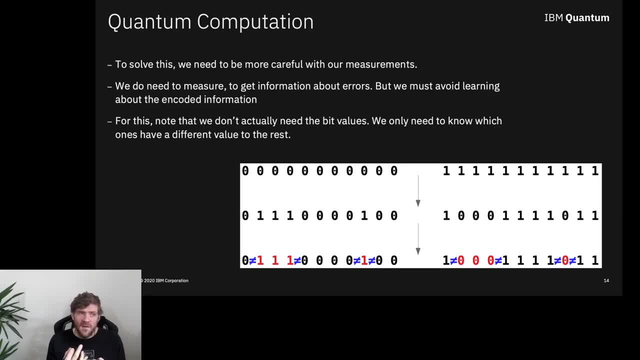 to get their values, but some sort of joint information about relationships between the bits. So let's look at an example with a lot more repetitions. Here we have a 0 turned into 0, 0, 0, 0, 0,. 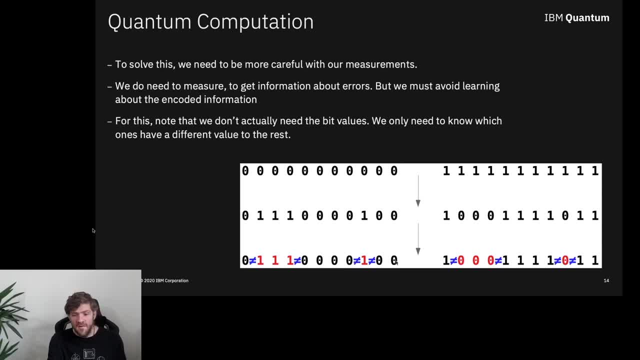 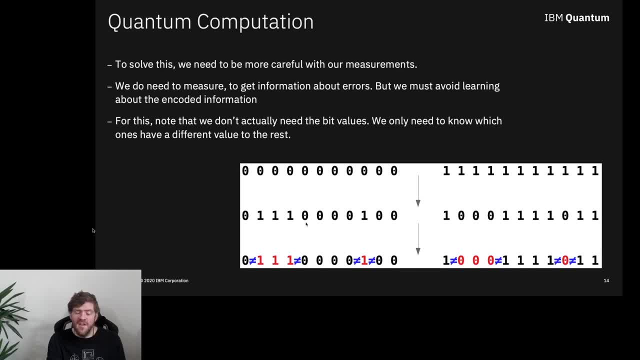 well, okay, this is initially our initial 0s. Then we have some errors. So we have errors occur on this set of three bits over on the left, and then there's one bit more towards the right, And here we're comparing what happens. 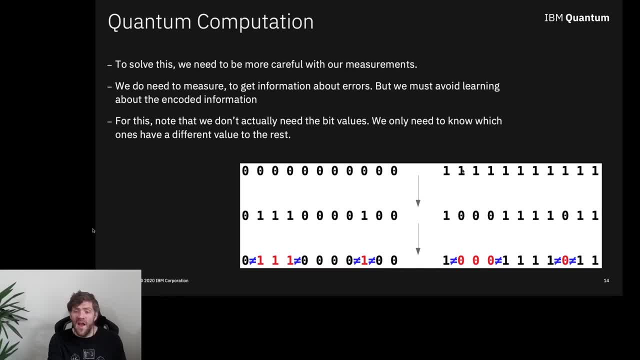 both in the case that we encoded a 0 and in the case that we encoded a 1, but with the errors occurring in the same places. So if we looked at those bits to see what they were, we would soon see that there are a few of them. 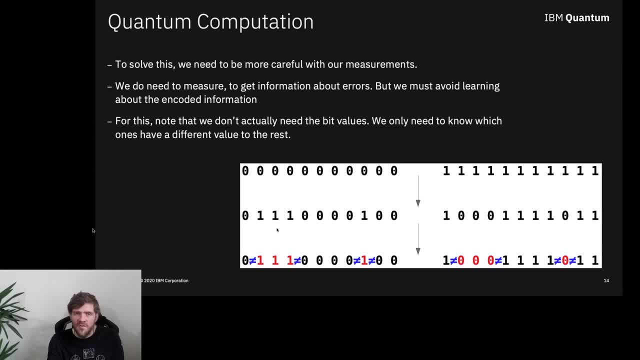 that are not in accordance to the majority, and we could guess that that might be the result of an error, but we would have also collapsed any possible superposition. But instead, what we could try to measure is the parity of pairs, So we could look at any pair of these bits. 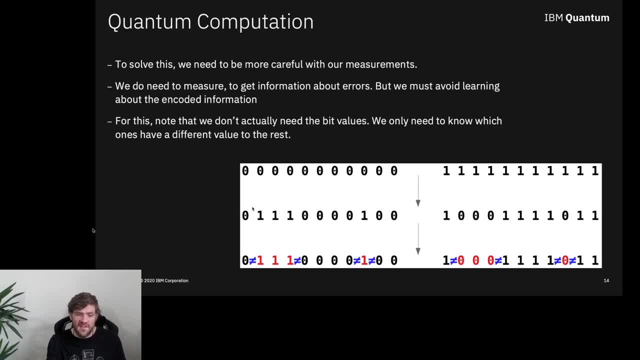 and ask: are they the same or different? So in this case we'd look at these and then we'd say, well, they're different. So that's why there's this blue non-equal sign down here. We look at the next. okay, they're the same. 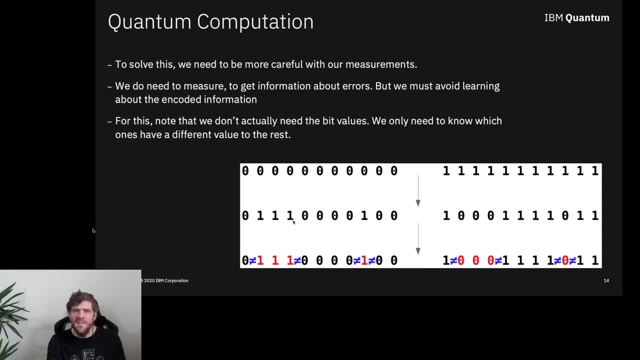 We look at the next pair, they're the same. We look at the next pair, they're different. And so we can continue that and look at that information of same or different between different pairs. And this is going to be the same for an encoded 0 as for an encoded 1.. 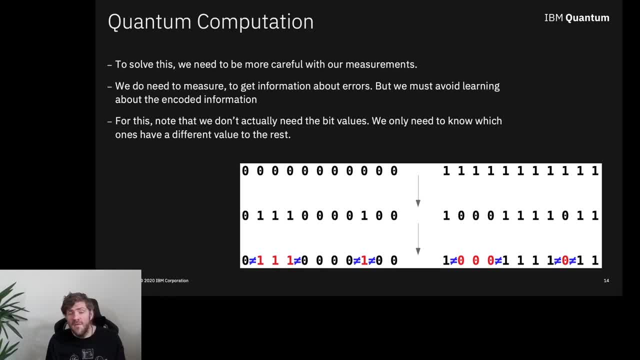 So this is giving us information about the errors, but it's not giving us any information about what was encoded, because this same or different information is completely the same, no matter what was encoded. But with this information we can determine where the errors were, because these not-equal signs 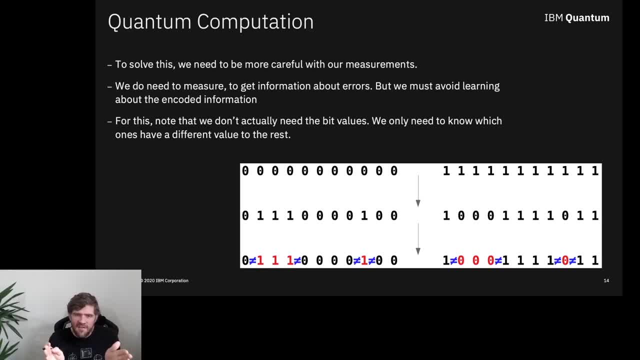 form the walls of the areas, of the domains where the errors occur. So these three flips are enclosed by these two not-equal signs. This single flip is enclosed by these two not-equal signs. So there are little flags telling us a set of errors begins or ends here. 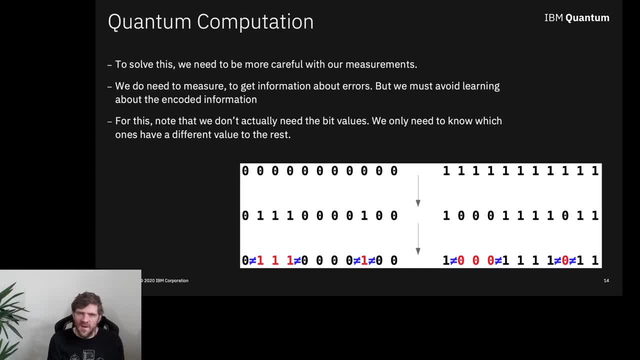 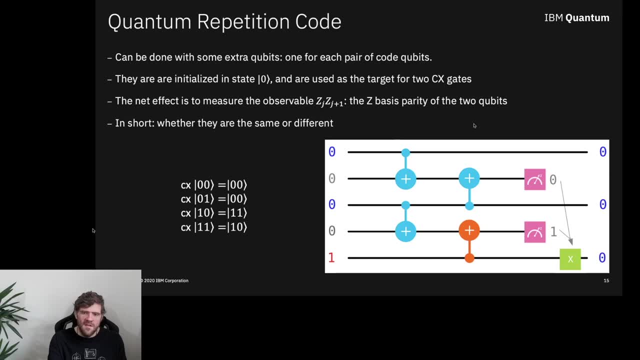 And so by looking at all of those, we can determine where the domains of errors are And we can correct them. So how do we perform these measurements? How do we get this parity information about pairs of bits or pairs of qubits, So this can be done with some extra qubits. 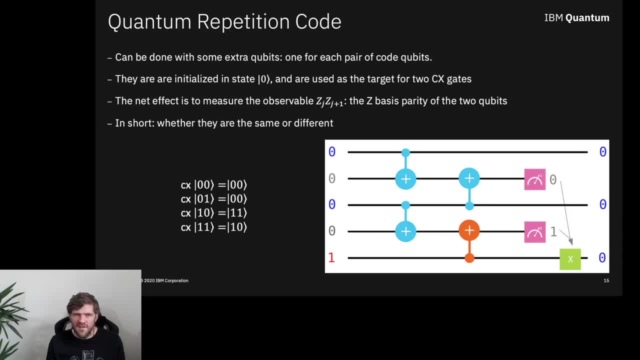 And here I'm kind of switching between talking about bits and qubits, because I'm talking about basically a classical error-correcting code and thinking about how to encode it on qubits. So they're a little bit interchangeable at the moment. So we can do this with some extra qubits. 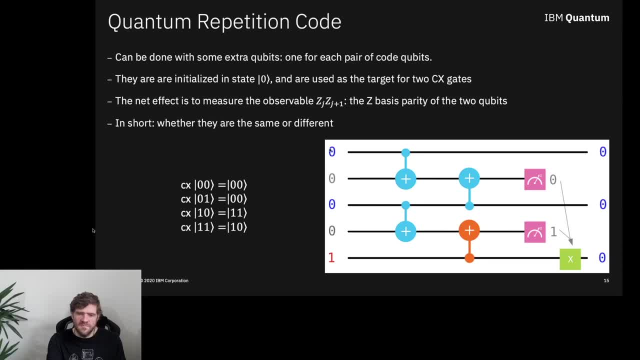 So here, the blue and red bits, or qubits, that are on this diagram represent the ones that we are using in the code. So they are 0,, 0,, 0 if we're encoding a 0, and that's what we see here. 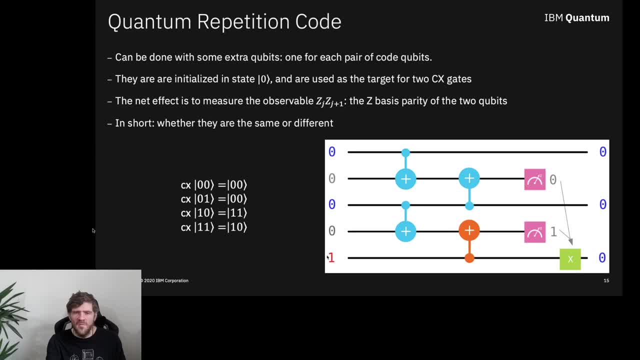 There would be 1,, 1, 1 if we're encoding a 1,, although the red one is the opposite value because it has been hit by an error. The two grey qubit or bit values are some additional ones which are always initialized in the 0 state. 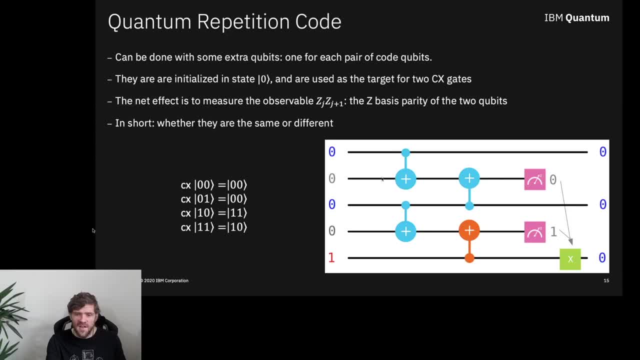 And then we perform some controlled knots. So if we take this controlled knot up at the top here and then the next one down, what they are doing is flipping that extra qubit, the qubit between that pair. They are flipping it depending on the value. 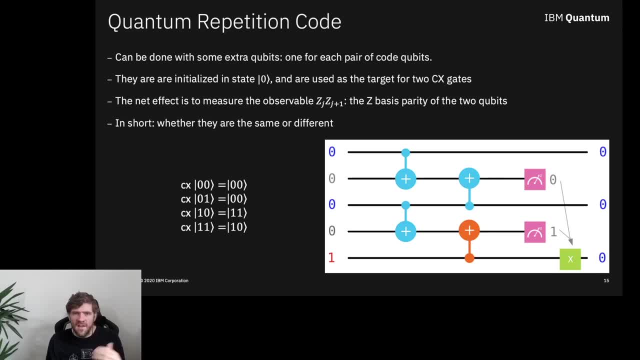 of the bit used for the encoding. So if we have a case, as we have here, where both of these are in the state 0, then neither of those will flip that middle bit and it will come out 0. If we have the case where they're both 1. 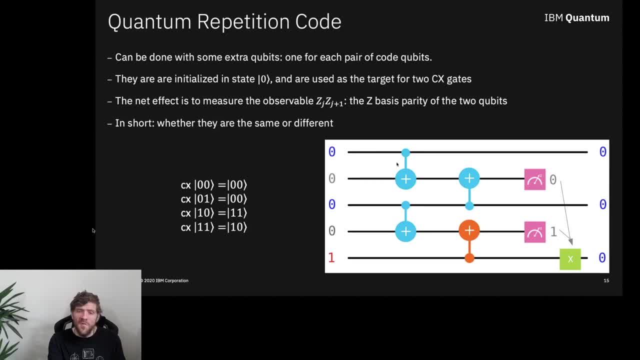 because we're encoding a 1, then both of those will flip that middle bit, flipping it from 0 to 1, but then back to 0 again. So in that case it's 0. So in the case that those two are the same, 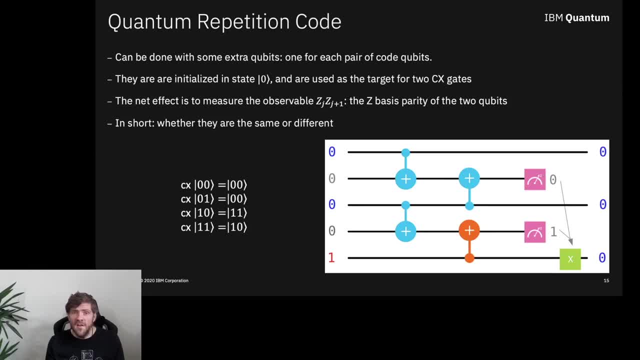 the middle bit, or qubit, will be measured and give an output of 0.. So 0 means they're the same, But if they are different, then one of those will flip it and the other one won't, and we'll get an output of 1.. 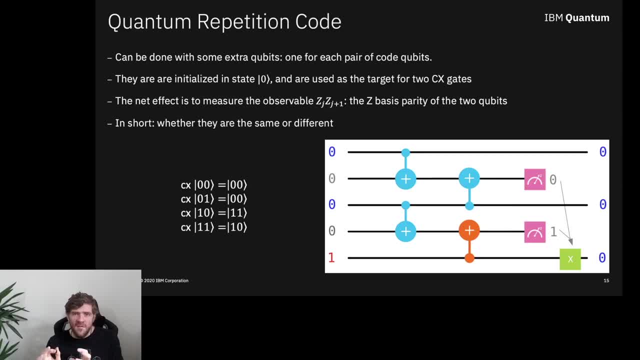 We don't get any information about which was the one that was responsible for flipping it. We just see that one of them is different from the other. So we get information about the parity without learning any information about what the values actually are. So this is what we need. 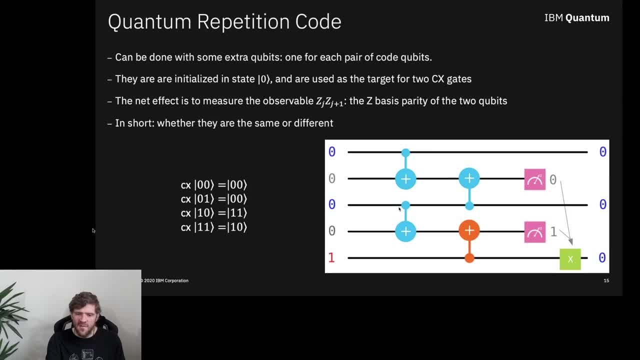 So in the bottom one here, because we have a case where one of them is 0 and the other one is 1, then the extra qubit is output as a 1. And so by taking that information in this particular case, 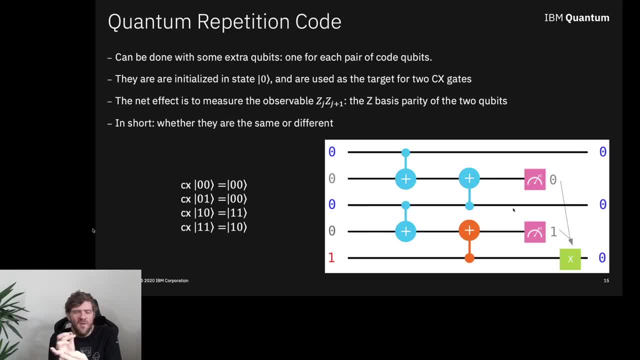 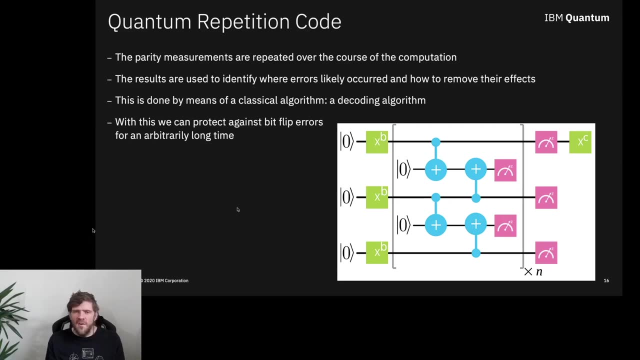 we can deduce that there's a barrier over near the end, and so it must be that end qubit. that is the one that was incorrect, So we correct it by doing another flip to flip it back. So these parity measurements are repeated over the course of the computation. 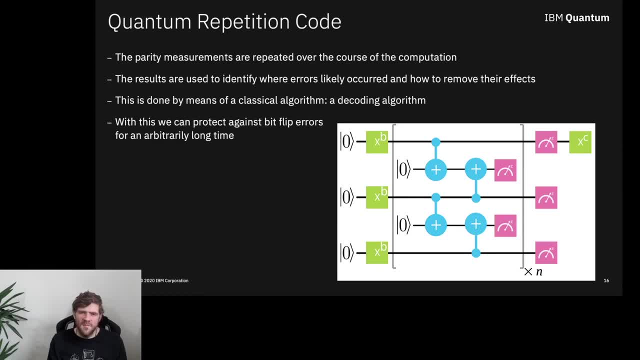 and the results are used to identify where the errors are likely to have happened and remove their effects. And this process of looking at these values and thinking, well, what could have caused this? What was the error? in this case, It's done by the decoding process. 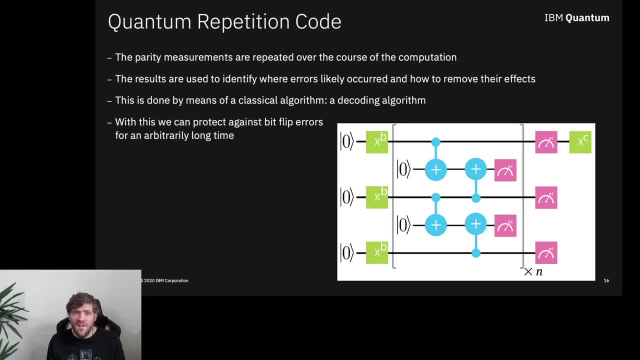 So the decoding process here is not trying to get the message out, It's just looking at the hints as to what errors occurred and use that to determine how to correct the errors. And by repeating this process many times, of extracting this information and using that to correct what's happening. 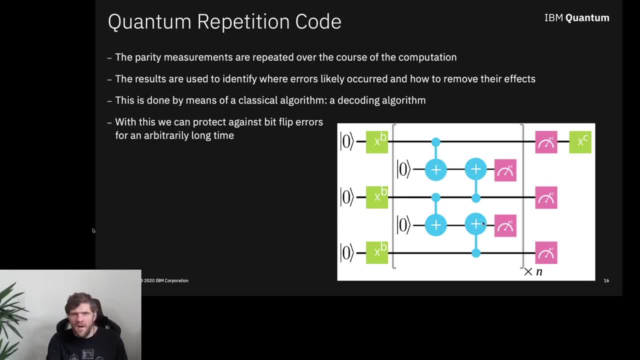 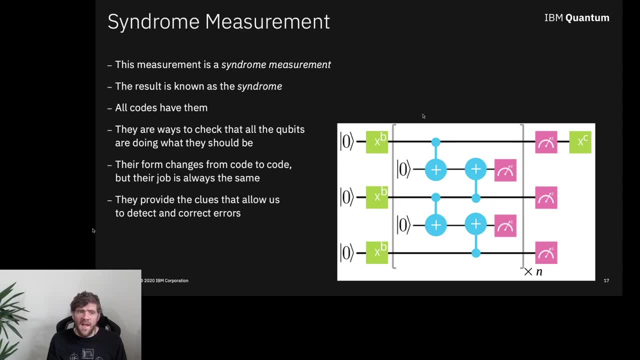 we can protect against bit flips for an arbitrarily long time. So this process is known as syndrome measurement and the result is known as the syndrome, And so all codes have some form of syndrome measurement, and they're often assisted by auxiliary qubits, as we see here. 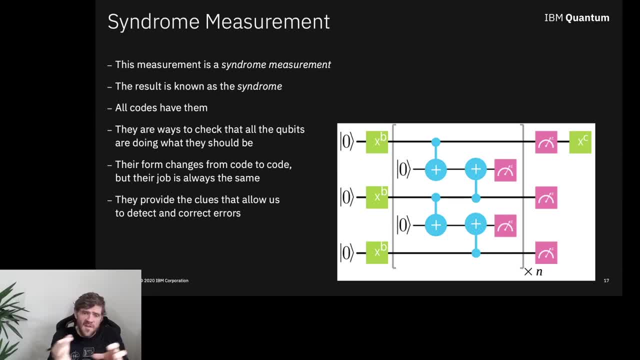 where we sort of use controlled operations to move the information about these hints as to whether or not errors have occurred onto the auxiliary qubits and then measure those. It's not always quite like that, but this is often how it's done. So they are. 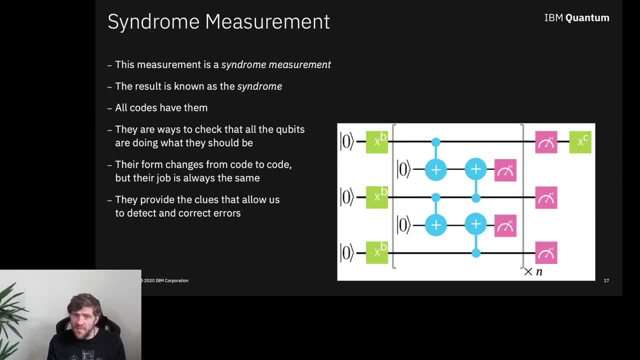 so they are used to check that the qubits are doing what they should be, And they typically have a value that they take which is typically zero, telling you everything's good, Whereas if they take a different value, typically one is telling you. 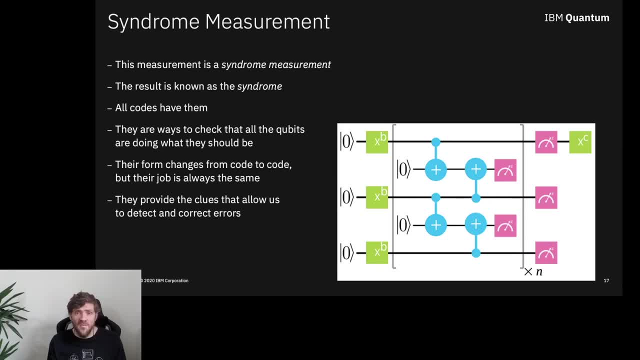 warning, warning. some sort of error happened, And then you have to look at all of the syndrome to try and deduce where that error happened. Yeah, so they provide us the clues and we have to solve the puzzle about how to correct the errors. 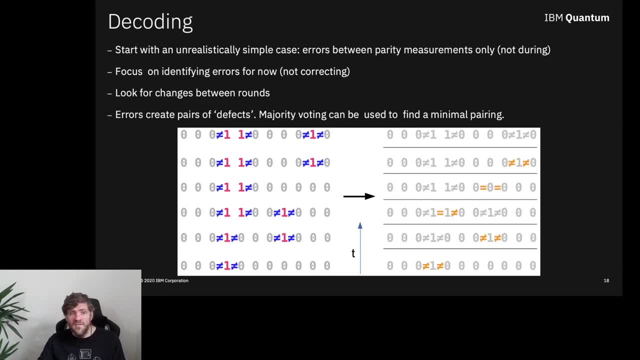 So, for an example of decoding, let's start with an unrealistically simple case, which is that errors occur between the parity measurements only and not during the parity measurements, So that we do all the parity measurements. that tells us some information, And then we have a moment. 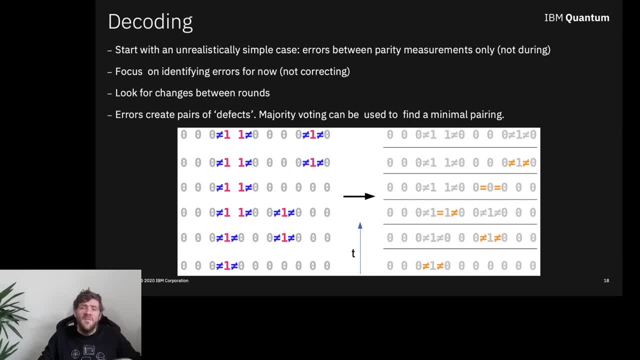 where errors can come and prod things. And then we do the parity measurements again, And so each time we do the parity measurements it tells us some information. So here we have time going from top to bottom. So in the bottom row in this example. 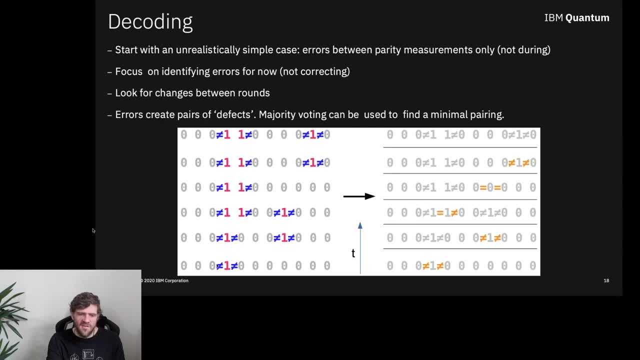 we see an error happening and it causes these two parity measurements to tell us something is wrong. Now let's suppose we're just compiling the information. We're not doing anything with it at that point. So in the next time step then we're still going to see that those two 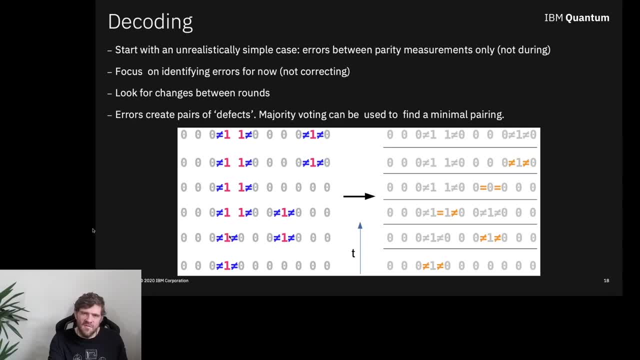 are flagging up that something is wrong because we haven't corrected it yet. But now there's been a new error Which flags up something is wrong And then in the next round another of the bits flips and this moves one of these things. 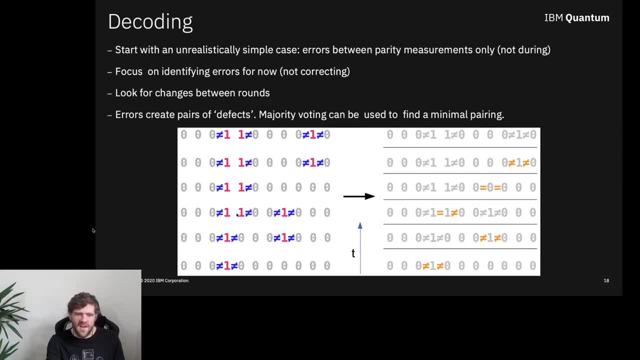 that's telling us something is wrong, Because now these two are no longer different. They are now the same because that error has been joined by another. So how can we correct this? Well, one way is to simply filter out what has changed between each pair of rounds. 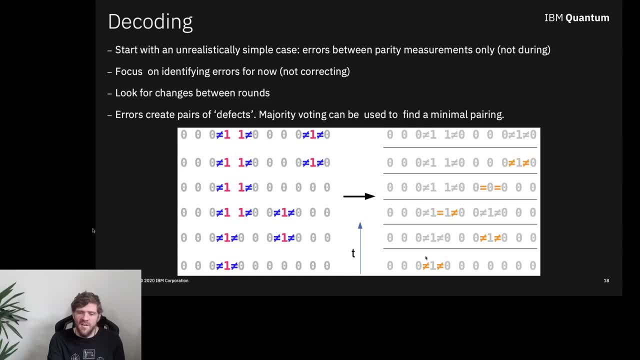 to see what new errors have occurred during each pair of rounds. So here: we initially expected everything to be fine. These two weren't fine, So that's new, and we flag it up The second time. these two say something's wrong. 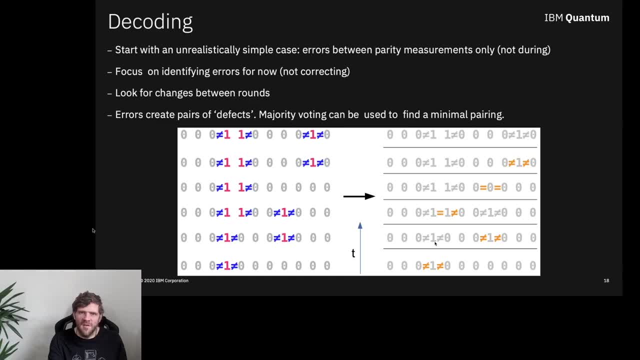 But we already know that They should still be telling us something's wrong. At that point, then, telling us something is wrong is what we expect, And it's not a signal of any new errors. But these two we didn't expect. 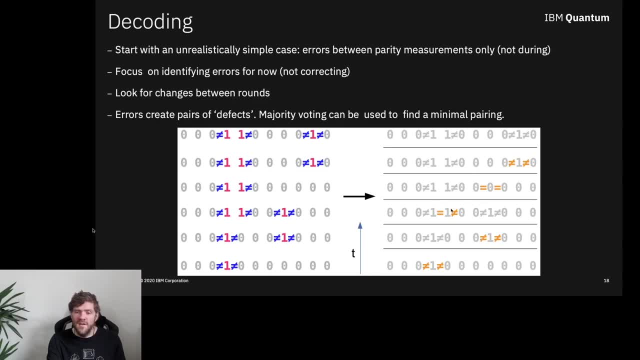 So that is something to take into account In this case. we did not expect it to tell us something was wrong here, But we also did not expect it to tell us everything was OK there. So in that case, telling us everything's OK. 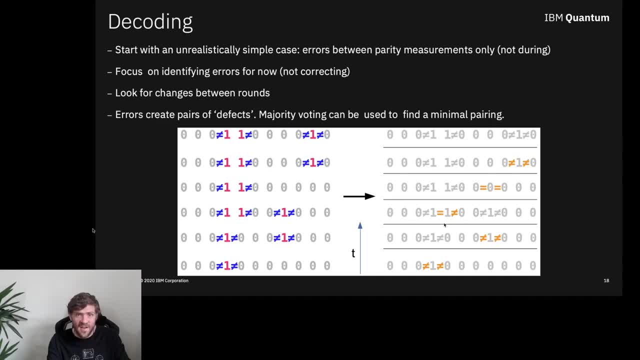 when we expect it to be. telling us that everything's not OK is a signature that something different has happened, Some new error has been introduced, So we flag that In the next one then. Oh yes, So in this case there was a bit flip. 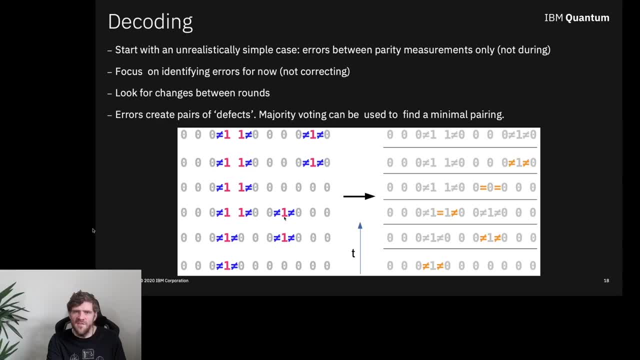 that caused an error here And it persisted for a little while, But then it was hit by another bit flip, So the errors corrected themselves. But from our perspective, we were expecting to see an error here And we didn't, So now we flag that up. 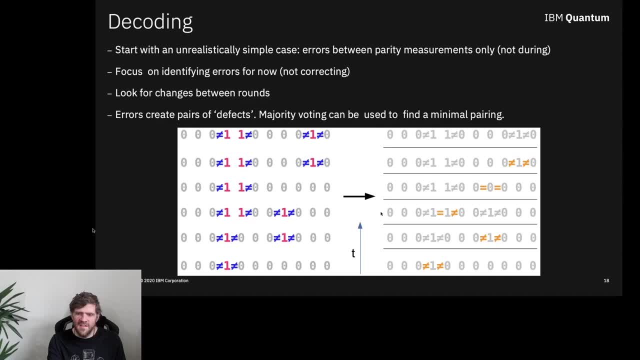 And so on. And so now in each case it's a pretty easy decoding process because we just have these pairs of things saying something weird happened around a single bit, And so we can say, oh well, there's a bit flip there. 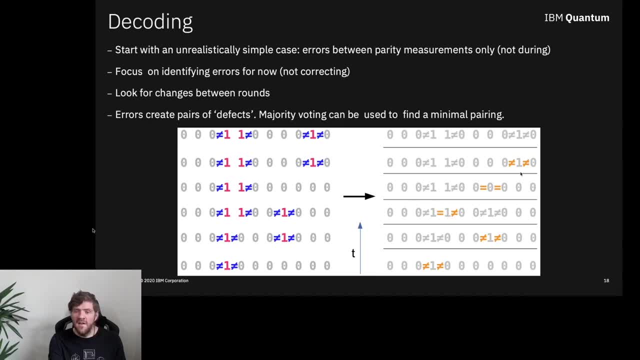 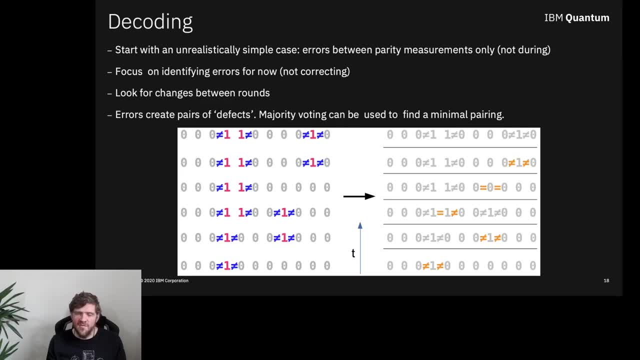 we can use a majority voting, where we use these domain walls to split everything into two domains, see which domain is the bigger one and assume that that was the one that didn't get hit by errors, And then assume the smaller one is the one that did get hit by errors. 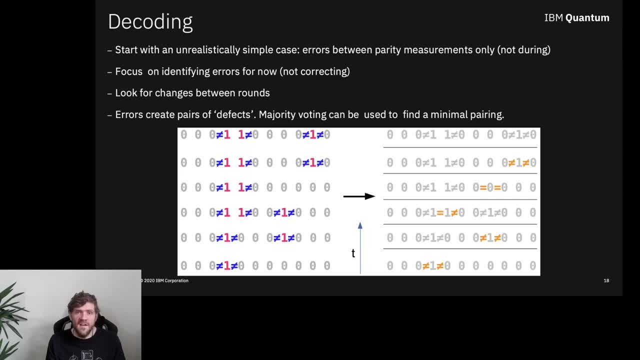 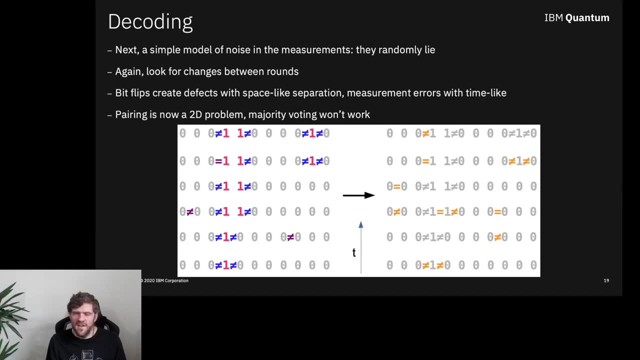 Because errors, hopefully, are relatively rare. Now, if we have another simple model of noise, but one in which it's a little bit more complicated, we can say that the measurements could randomly lie. So when we make a measurement it doesn't give us the true result. 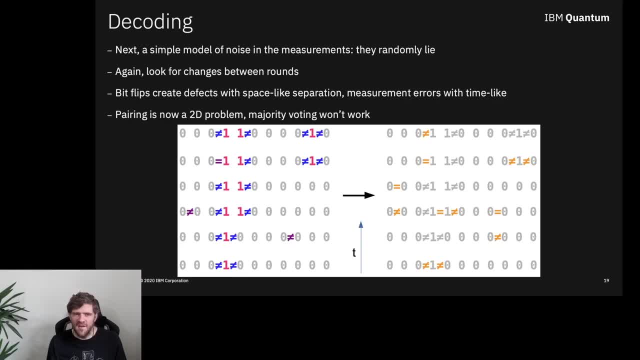 all of the time, There's some probability that it's incorrect. We can again look for changes between measurement rounds. So here, we didn't expect these two, So that was a change. Here, we did expect them, So that wasn't a change. 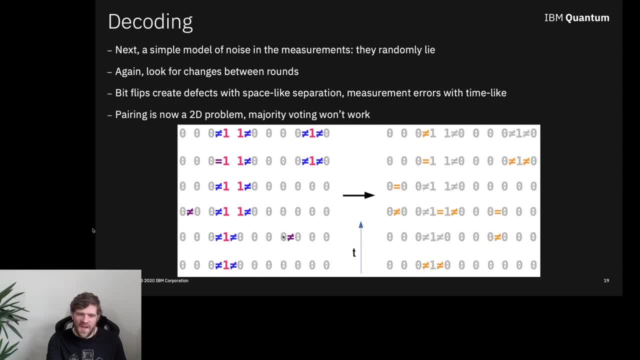 Here we've just got one pair of bits telling us that they are different in the middle of nowhere. Well, that's weird, So that's something to flag up. And in the next round it tells us: oh, they're not different after all. 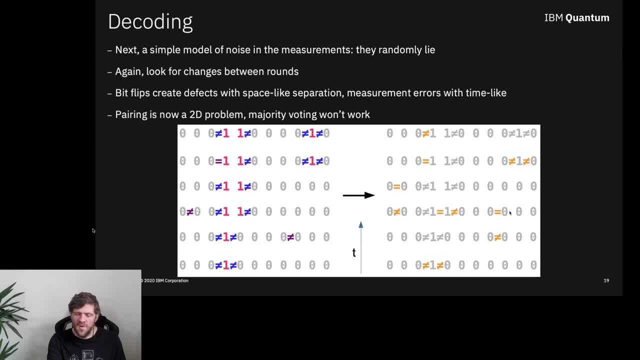 And so it does that forever more as well. Okay, well, we expected to see something there And we saw the wrong thing, So we flag that up, And yeah, so on and so forth. Well, what we're seeing in this case? 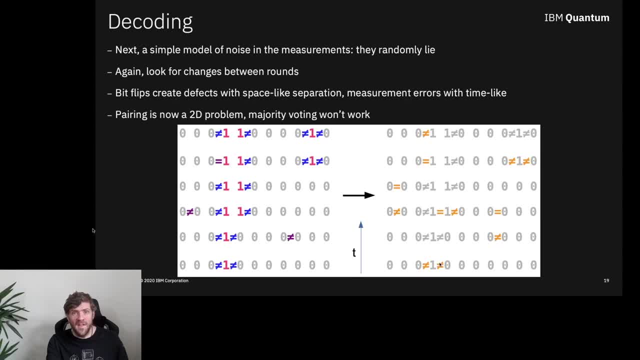 is that? well, when we have errors on bits or qubits, when we have bit flip errors, then it's causing a pair of these things to be flagged up horizontally. But this case was probably just our measurement lying to us And that causes us. 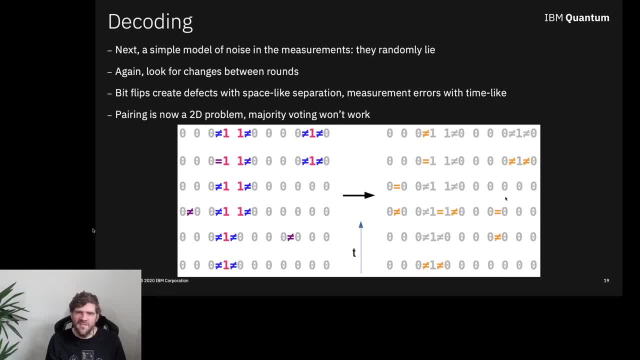 to have pairs of these little flags telling us that something has gone wrong, vertically, so in the time direction. So this is now a more complicated process for decoding, where we don't just do lots of majority voting but we've got to look for pairs of hints. 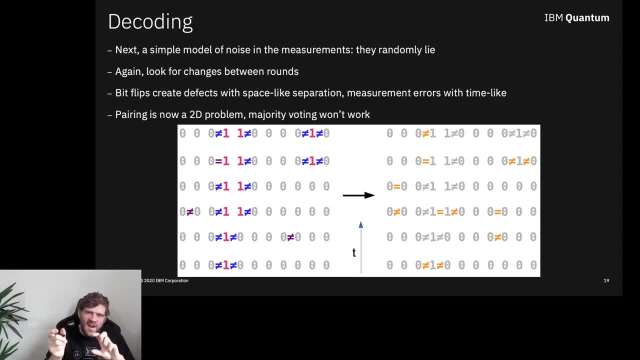 which are going to be oriented in any direction in this two-dimensional space caused by the action of the code and then also time. And when we look for surface code decoding later, the surface code is going to be more of a two-dimensional object And then, by adding in time, 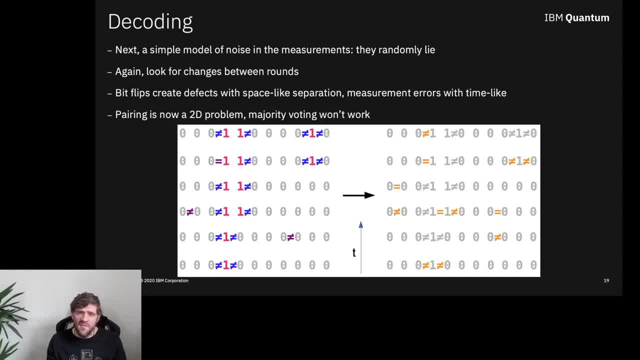 we have a three-dimensional decoding process, But it's going to be very much the same algorithm that we actually use, So there are many ways to try and take this sort of two-dimensional information about weird things happening and try and work out what error occurred. 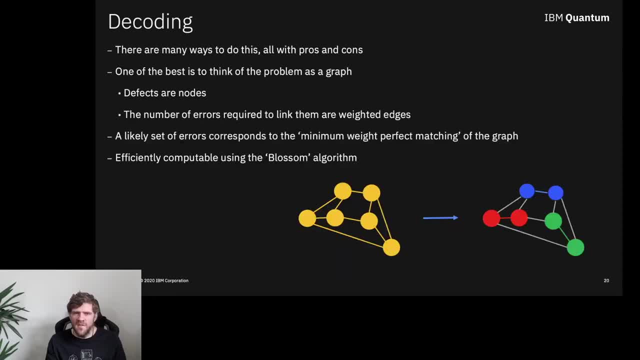 With different pros and cons, But often the best way is to think about it as a graph where the defects are nodes and the number of errors required to link them are weighted edges, And a likely set of errors corresponds to the minimum weight-perfect matching of the graph. 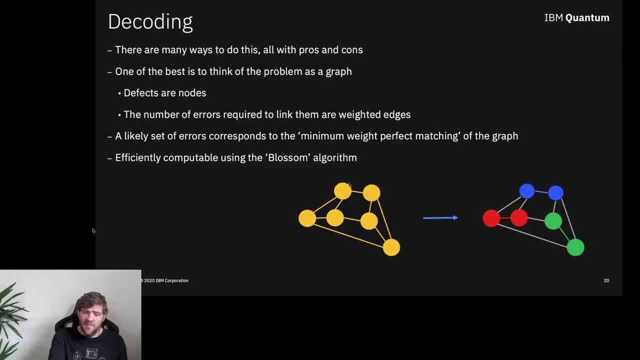 What is a graph? at least in the mathematical sense? It's a collection of nodes and edges, where the edges connect the nodes, and then we can pose all sorts of mathematical problems based on this. And one problem is: given a graph, is it possible to find a perfect matching? 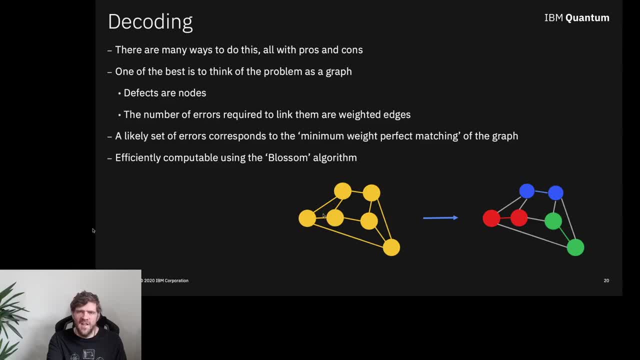 So a perfect matching is a set of edges where each edge touches one and only one node. So for this graph we have here, here is a perfect matching where we keep this edge which connects these two, We keep this blue edge which connects the two that have now been coloured blue. 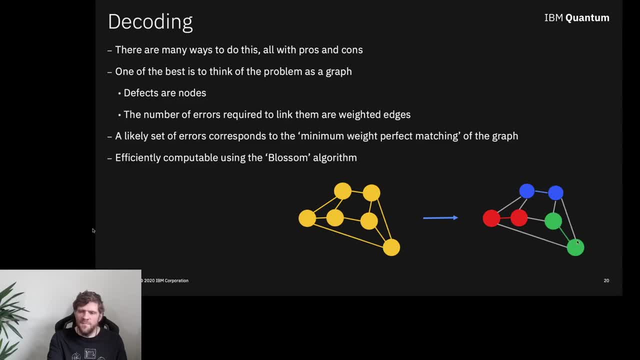 We keep the green edge, which connects the two that have now been coloured green. Every node is touched by a single edge, and so we've found a matching which is essentially a pairing of the nodes, such that the paired nodes are connected by an edge. 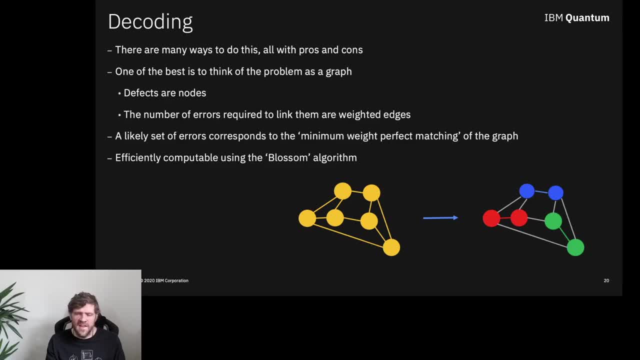 Now, a minimal weight-perfect matching is where we assign a number to each of the edges and so for a matching, we add up all of the numbers of the edges that are included and we want to find a perfect matching of minimal weight. So let's see why we might do this here. 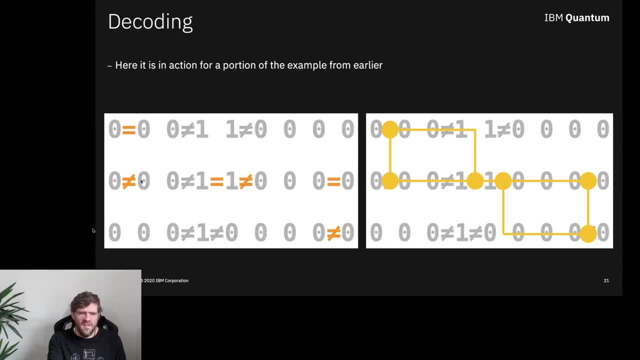 Well, we can think of these hints that we've got in orange as our nodes, and we can think of there being edges between these nodes when it is possible for some error to have caused both of those. So if we think of these two orange ones here, 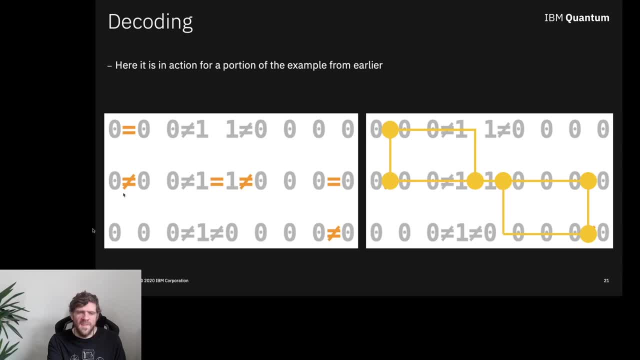 and we think of them in complete isolation. then what error could have caused us to have these two flags, one after the other? Well, it could have been caused by a single lie in a measurement error. So, for those, we connect them by an edge, because it's possible to have performed an error. 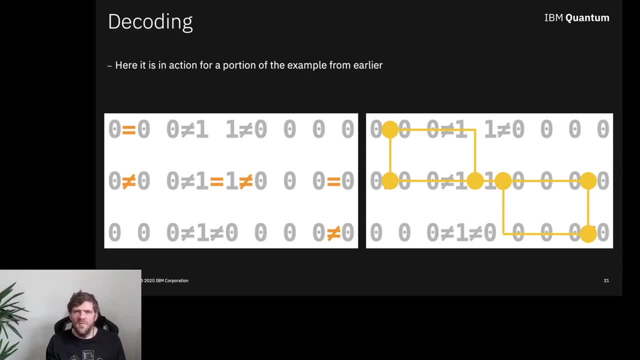 which caused both of those in isolation, and we give that edge the weight 1, because only one error would have had to happen, Whereas for this one and this one then it is possible an error could have caused those both to happen in isolation, which is to have flipped the three bits between them. 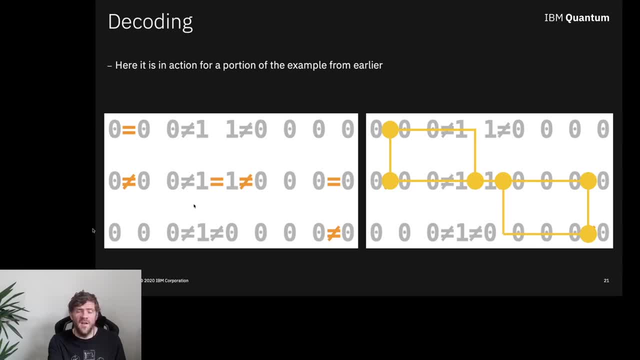 but that requires three errors. so we give that a weight of 3.. So here we've got an edge with a weight of 1, here we've got one with a weight of 3.. Now, if we were to think about this one and that one, 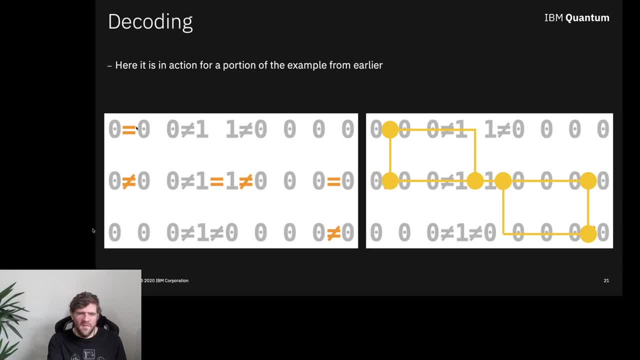 then what would have had to happen here? Well, we could have a node here and here created in isolation, if we had three bit flips between them and if there was a measurement error causing this one to have registered the wrong result, that could have made it seem like 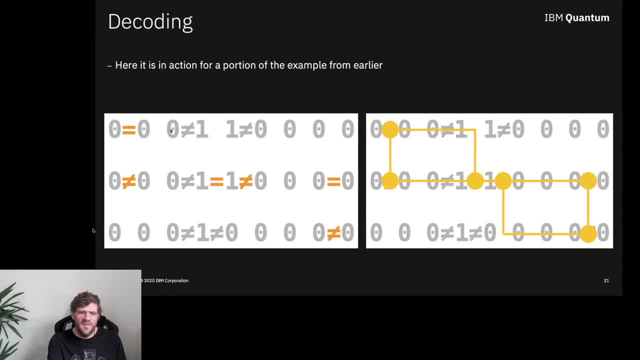 it occurred a little bit earlier. So we would need three errors on actual bits and one measurement error to cause these two to occur in isolation. so we can assign that a weight of 4. Or we might choose to change our weight a little bit if the probability of a measurement error 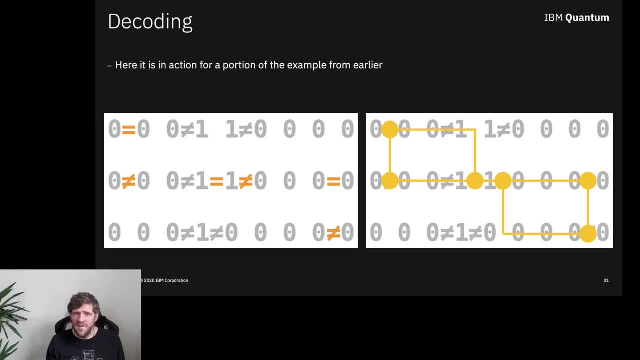 is much more or less likely than the probability of an error on a bit, then we might use that information in defining our weight. But let's just use the number of errors so far. So that would be a weight of 4.. For these two it would be a weight of 1. 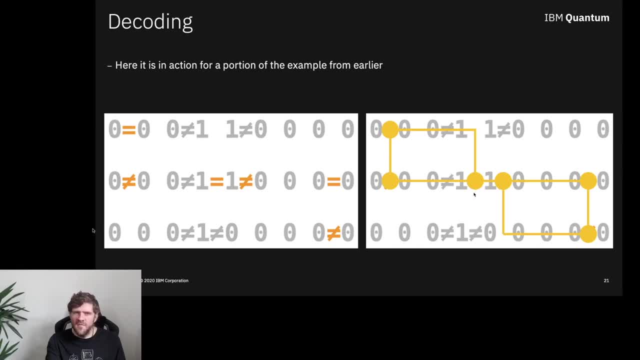 and so on and so forth, And then a matching of this would be a single set of errors that could have been responsible for the whole thing, And by choosing the minimum weight matching, we want to find the smallest number of errors that could have caused this. 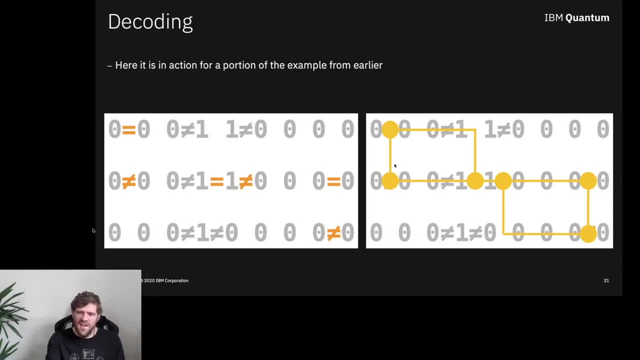 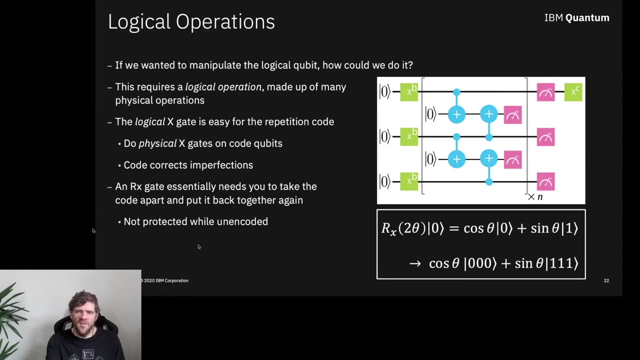 And so just having a single measurement error here, a single measurement error here and a single bit flip error here would be that minimum weight, perfect matching, And there is an algorithm to find these, so that's awesome. Okay, now let's move on to logical operations. 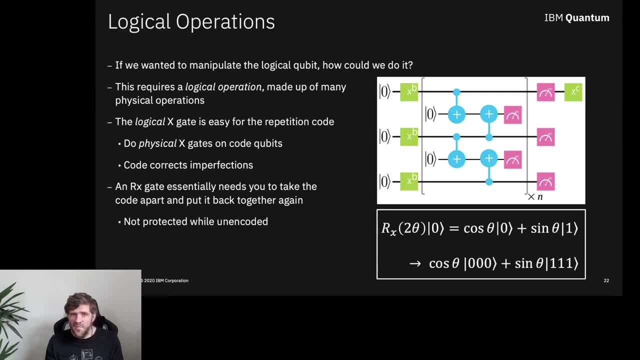 We've found a way to do an encoding which doesn't destroy superpositions. It can find bit flip errors. We can use decoding to try and work out exactly where those bit flip errors were in order to take that information into account. But it's not just about protecting a qubit. 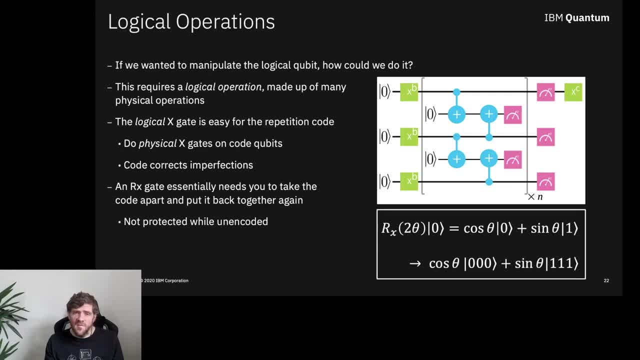 it's also about trying to do things with it. So how do we perform logical operations? These are gates performed on our logical qubits. Well, the physical- I'm sorry- the logical X is very easy for the repetition code because we just have to flip all of the repetitions. 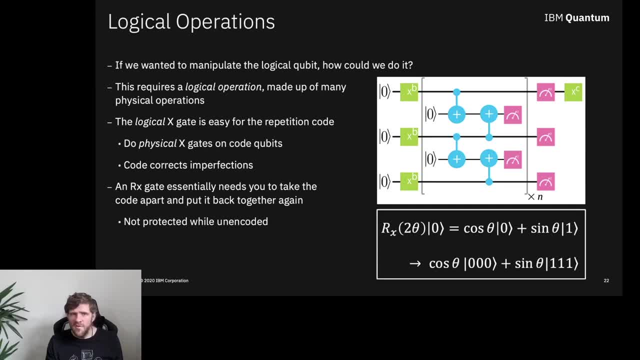 If we've got loads of zeros and we suddenly want them to be encoding a one instead of a zero, we just go and flip all of those zeros to ones. There you go, Job done. So if there is some imperfection in our X gates that we perform when doing that flip, 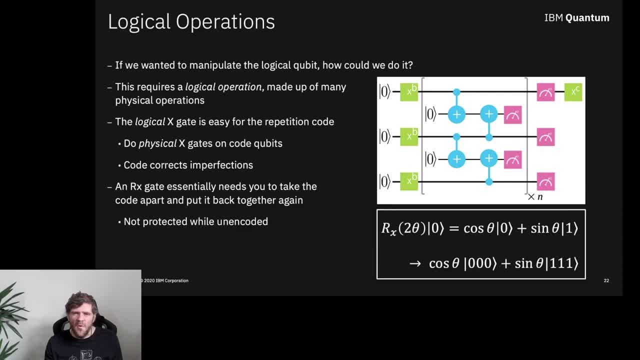 it just means that there is a little bit more error. So if we've done a load of syndrome measurements and then we want to do our logical X, and we do an X on all of those physical qubits and then we start doing syndrome measurements again, 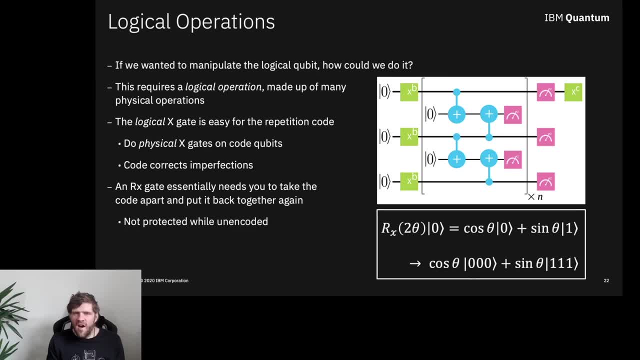 then we can expect the syndrome measurements after the logical X to be a little bit more likely to see errors, because there would have been some errors introduced by our physical Xs, but it can still detect them and correct them in the same way. So that's perfectly fine. 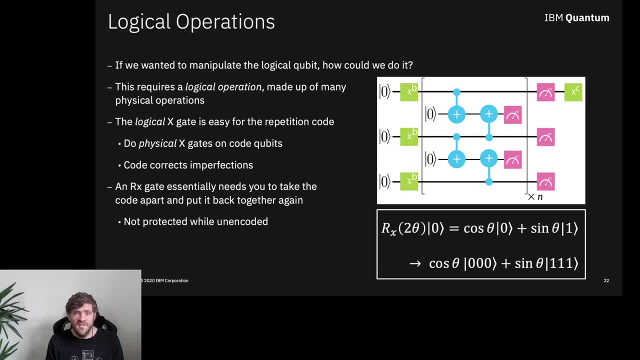 It's a logical operation which is consistent with our scheme for detecting and correcting errors, So the imperfections in it just get detected and corrected. naturally, It's all good, However, for something like a rotation around the X axis. and if you apply a rotation around the X axis, 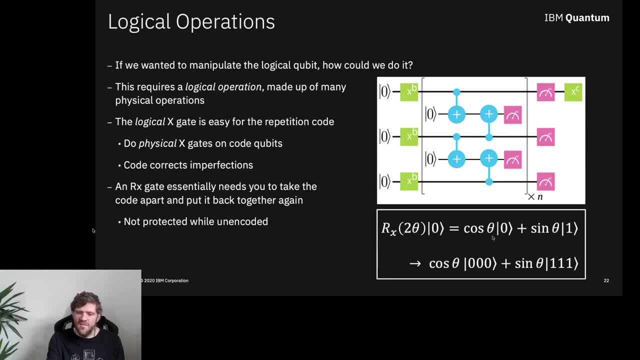 around some angle, 2 theta to the zero state. it will give you some superposition of cos theta 0 and sine theta 1, which encoded would be: cos theta 1, cos theta 0, 0, 0 and sine theta 1, 1, 1.. 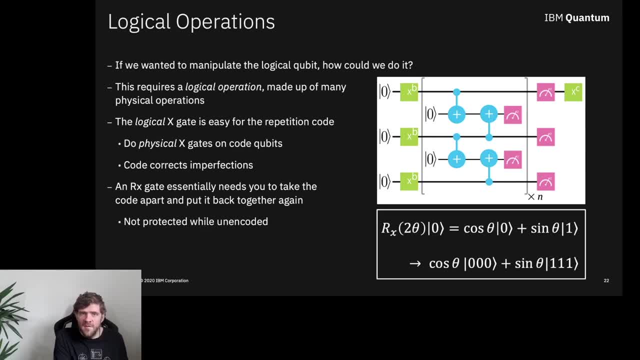 So to go from a 0 0, 0 to some superposition of cos theta 0, 0 and sine theta 1 1, 1, some complicated entangling process has to be performed there and that is not necessarily going to be nice and compatible. 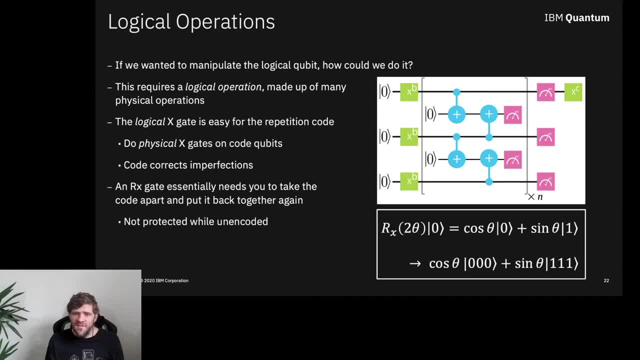 with the scheme we've got for quantum error creation, We're going to have to do some controlled operations between the qubits that are encoding the logical information, and that means that if there are some errors occurring on 1, those entangling operations might spread those errors around. 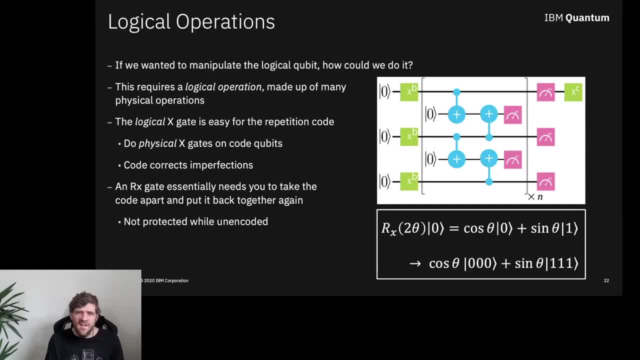 in ways that can't be nicely detected and corrected. So basically, we actually have to take the code apart, perform the rotation and then put it back together again, And so for that moment, as we've taken it apart and then performed the rotation, it's not actually protected. 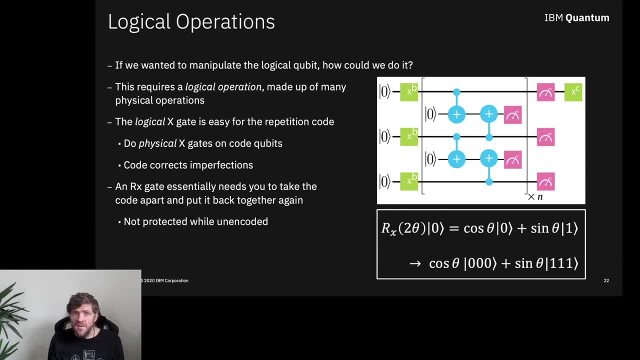 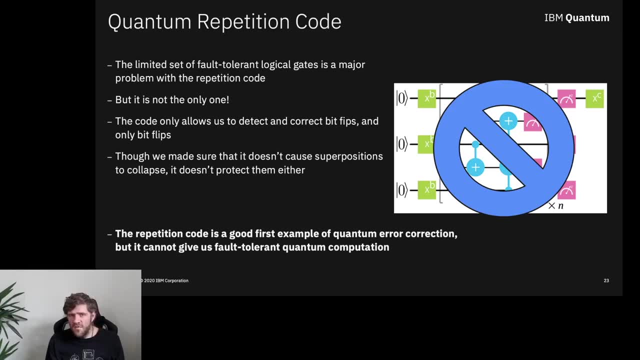 So we can't do this operation in a way that is fault tolerant using this code. So the limited set of fault tolerant gates is a major problem with the repetition code, meaning that we can't use it for universal quantum computation. It's not the only one, though. 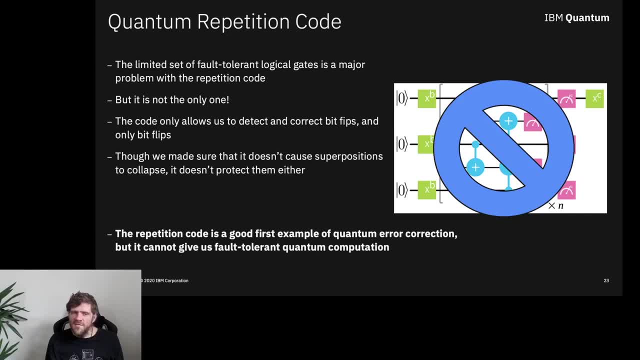 because it only allows us to detect bit flips and not phase flips. So we did add this additional feature, such that it doesn't destroy superpositions, but it doesn't protect them either. So if you've got phase flips in there, those phase flips are going to mess you up. 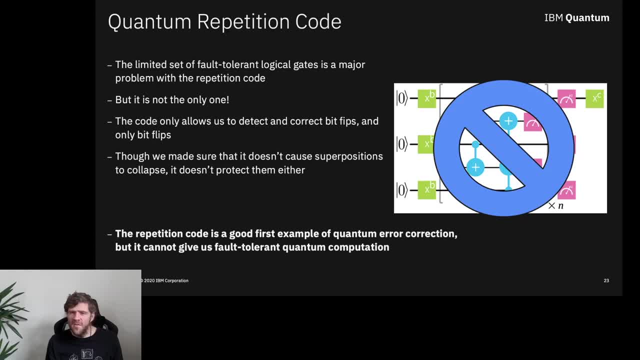 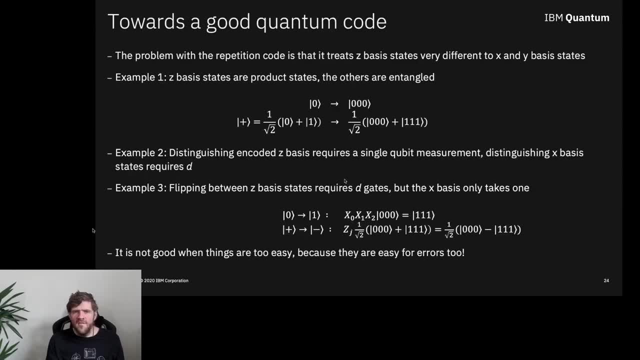 So it's a good first example of the ideas behind quantum error correction, but it can't give us full fault tolerant quantum computation. So what would we need to do to make a good quantum code? Well, the problem with the repetition code is it treats Z basis states very different to Y and X basis states. 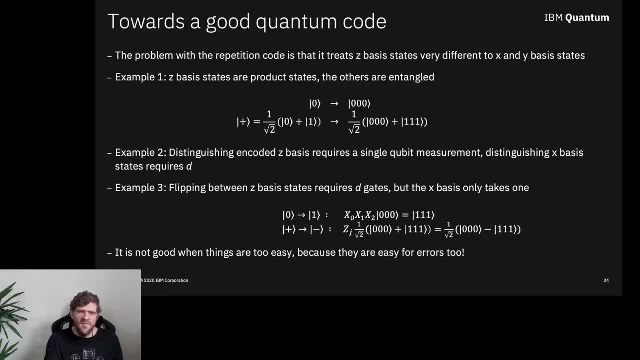 So, for example, the Z basis states are product states, 0 is just 0, 0, 0, 1 is just 1, 1, 1. this is for three repetitions, of course, but the plus state is a big superposition, a big entangled state. 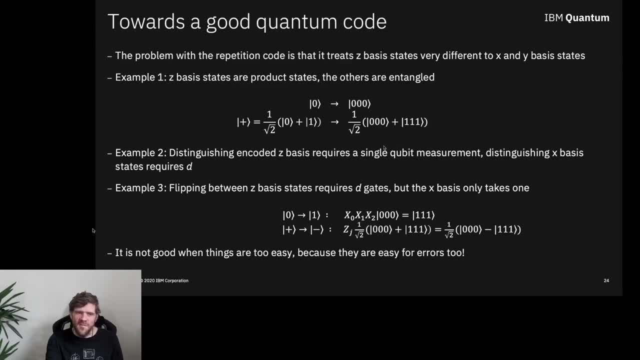 and so obviously that is quite a big difference between those two basis states. Also, if you want to distinguish between encoded Z basis states, then this is very easy, because distinguishing between encoded X basis states is a lot harder. So distinguishing between encoded Z basis states is making a measurement a Z measurement. 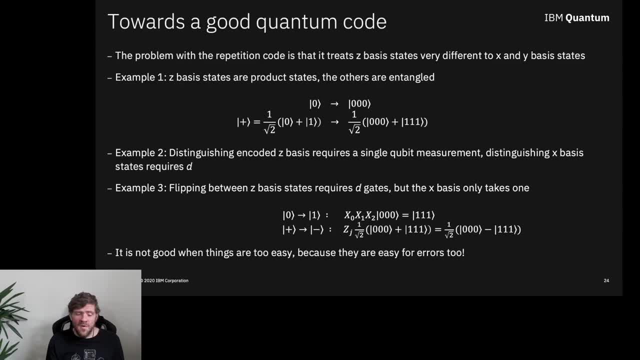 of the logical qubit. So how do we do that? Well, we've just repeated our information across a whole bunch of qubits, so we just look at one of them and that's fine. Of course, we should look at all of them and do some decoding in general. 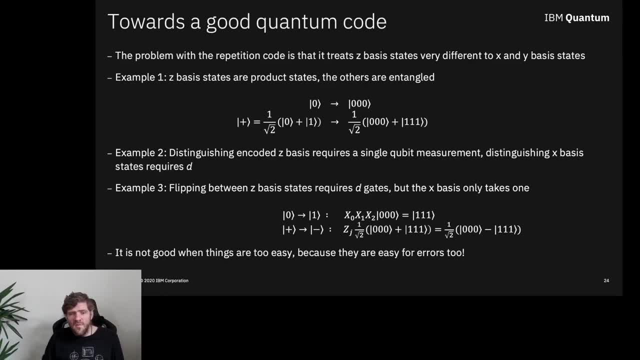 but in a perfect world you can just look at one. However, to distinguish X basis states you have to do something more complicated like undo the entire encoding and then look at one. And undoing the entire encoding means we have to act on all of the qubits involved. 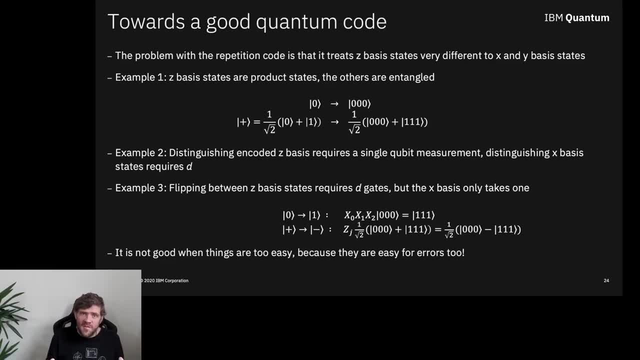 So there's a big difference in effort between measuring the X basis and measuring the Z basis. Also, flipping between Z basis states requires D gates. so from going from all 0s to all 1s you have to flip all of them. But to go from an encoded plus. 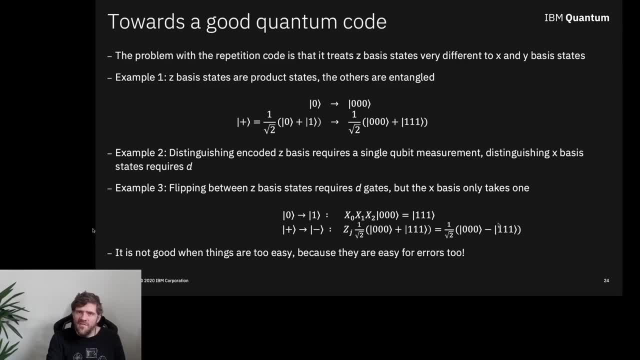 to an encoded minus. you can actually act on any qubit because every qubit has access to whether it's 0 or 1, and so if you want to flip between plus and minus state, which just means giving a phase of minus 1 for the state 1- 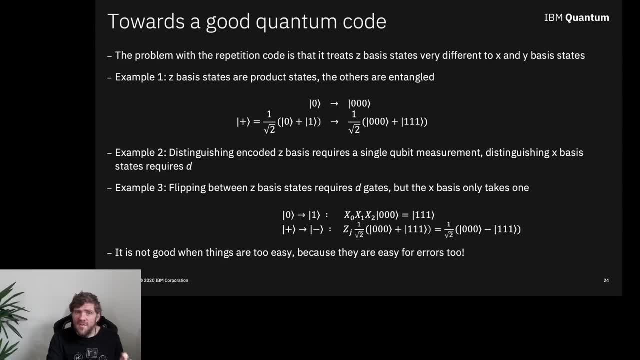 then you can do that on any of the qubits, So it's much more accessible. So, instead of having to do something to everything, you just have to do one thing and you can do it anywhere you want. So this is why we're protected against bitflips. 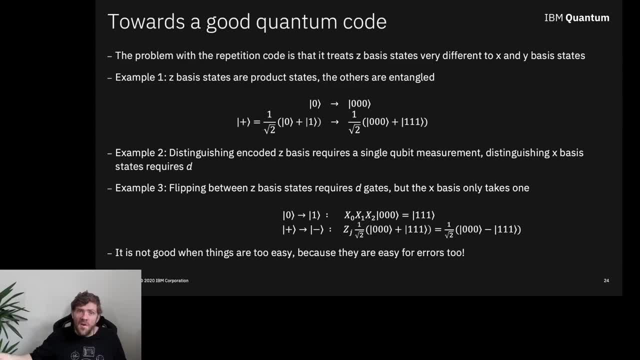 because you have to put in so much effort to do a logical bitflip, whereas to do a logical phase flip you can do that very easily, and this is why superpositions are so fragile in this code, because it has so many opportunities for errors to come and mess something up. 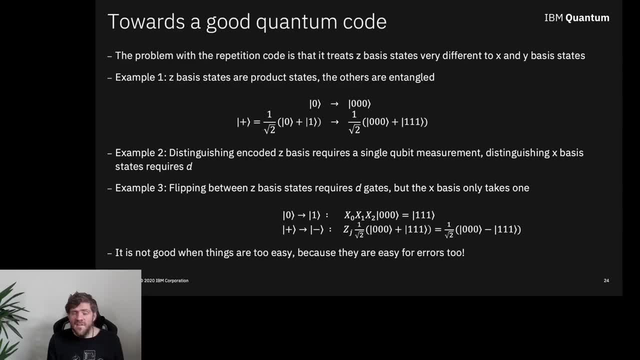 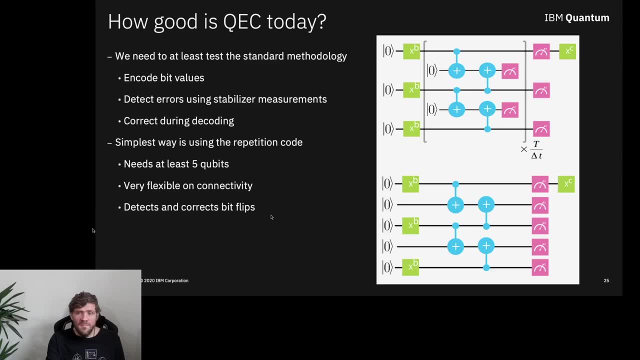 So these are things that we have to look out for when moving beyond the repetition code to a truly quantum code. So I'm going to finish off by giving you an example of where the repetition code is useful, which is in benchmarking, So we might not be able to use it. 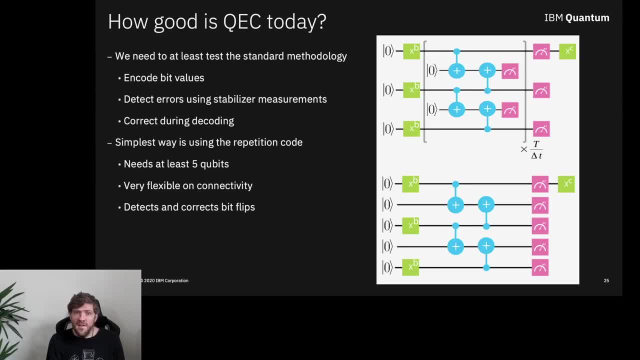 to actually protect our quantum information in universal quantum computation. however, it does test all of the standard things that we need, like encoding bit values, detecting information using, detecting information about errors, using stabilizer measurements, performing decoding. all of that can be done with the repetition code. We only need five qubits at most. 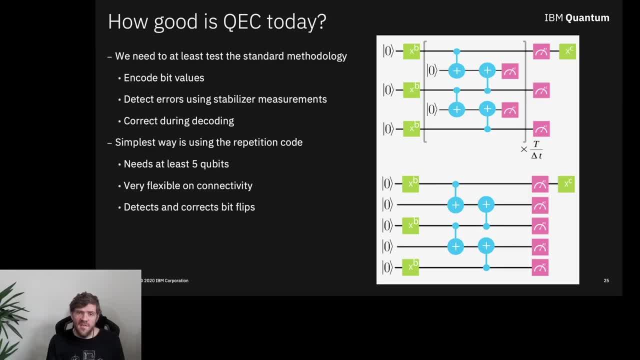 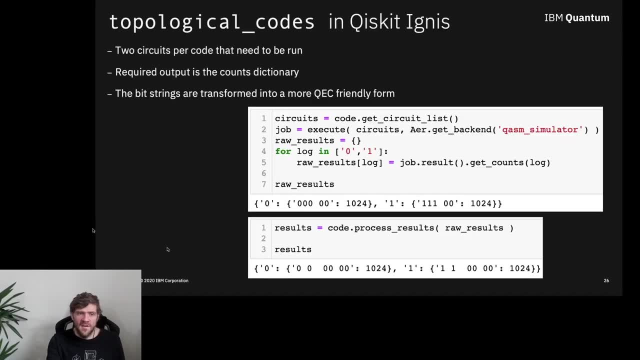 to do three repetitions and have the two auxiliary qubits to mediate the syndrome measurements and we can use it to detect and correct at least bitflips. So there's two circuits that need to be run per code in order to do some sort of test. 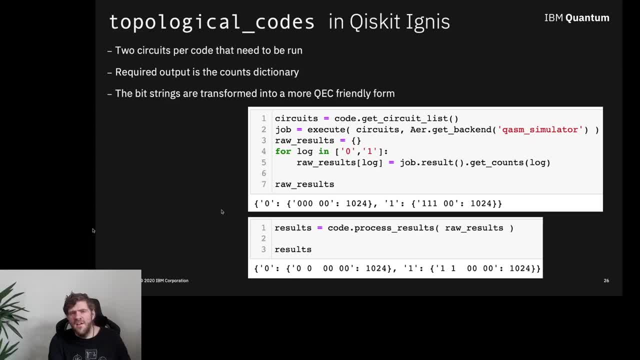 of how well it works, and we've actually got a tool in Qiskit Ignis which will do this for you and also transforms the bit strings that you get out as a result into a form that is more friendly for quantum error correction, which is basically taking the raw zeros and ones. 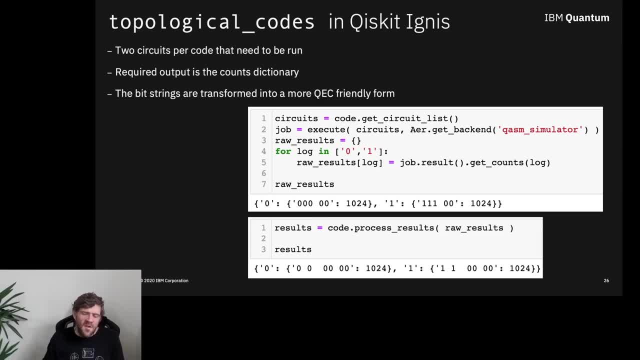 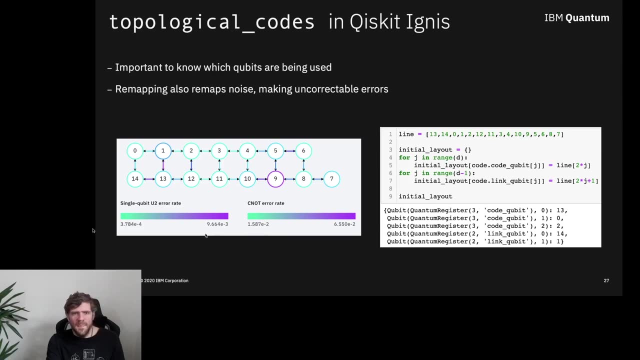 from all of the measurements and doing that technique of only caring when our syndrome measurement is telling us something new, in order to do the decoding much more easily. And when we're running this, it's important to know what qubits we're using exactly, because if the transpiler 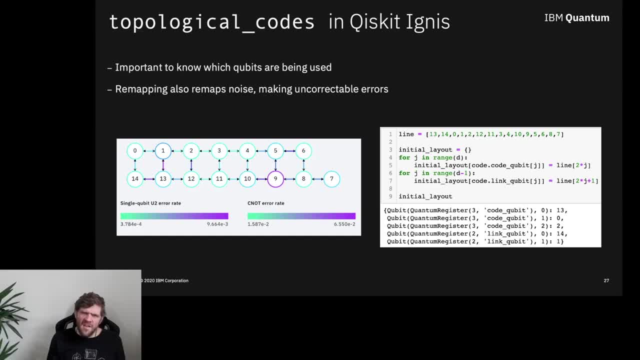 takes the circuit we've made and then says, well, how can I do that on an actual device? and induces loads of swap gates and stuff in order to make it run, those swap gates and stuff. they're all going to have errors of their own and they're also going to cause 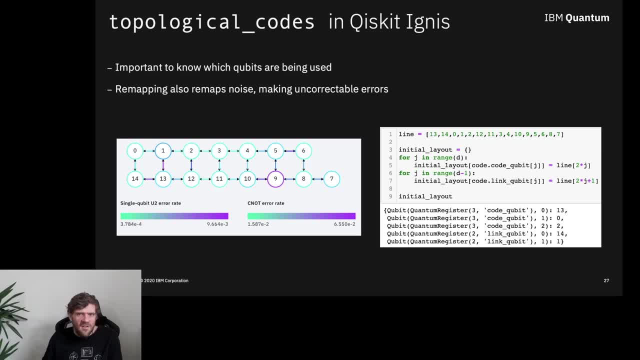 weird multi-qubit errors that are not of the form that we're really assuming, when we have shown that this code is actually good for stuff. So we have to think: well, I need a specific set of qubits in a particular order, so I need one to be the first. 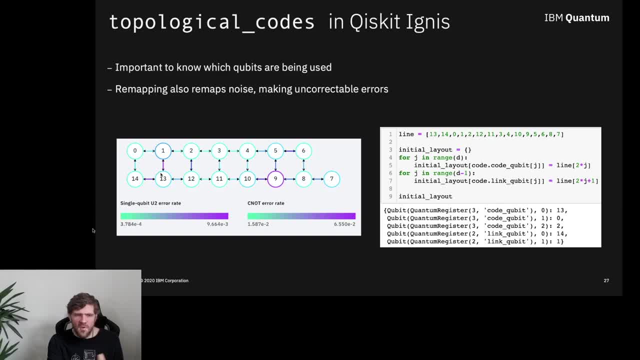 repetition of my encoded value. let's use qubit 13 for that. and then I need another one to be the auxiliary qubit, which is going to perform a parity measurement. I need to do a CNOT between those two, so let's use 14 for that one. 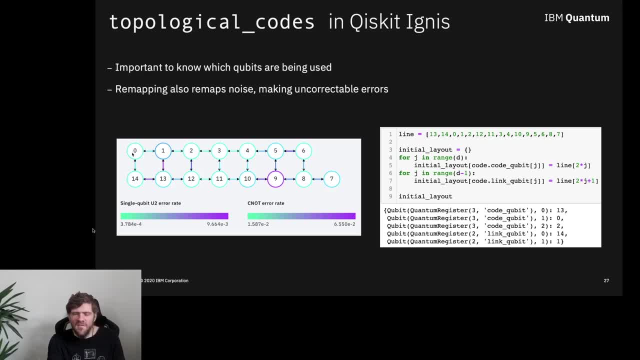 and then I need another one to be the other half of that parity measurement. so let's choose qubit 0 and then that's going to be involved in a parity measurement with another qubit. so let's say that's going to be involved with qubit 2. 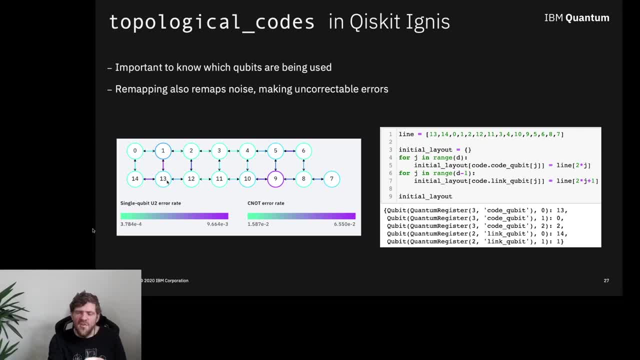 and their auxiliary qubit is 1, so I'm basically needing to choose a line of qubits, and so here I'm choosing 13,, 14, 0, 1, 2, 3, 4, 0, 1, 2,, 12,, 11. 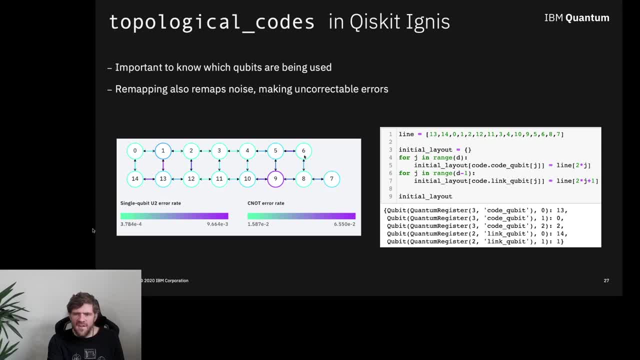 3, 4, 10,, 9,, 5,, 6,, 8, 7. Why such a weird combination? Just to show you that weird combinations are possible. and then in Qiskit you can specify an initial layout where you're saying specifically: 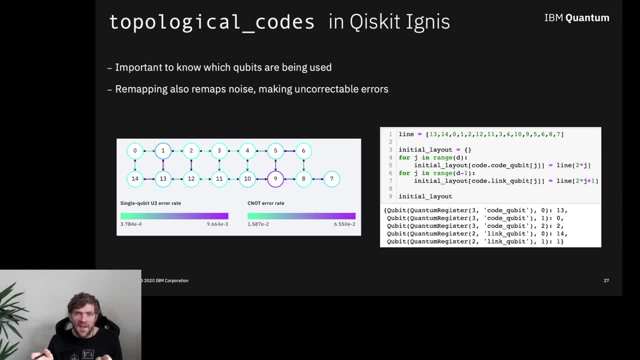 you should use these qubits for my circuit, and then the transpiler will see: well, can I run this circuit if I use these specific qubits, and it will see that it can, and then it won't bother with transpilation, which is going to mess everything up. 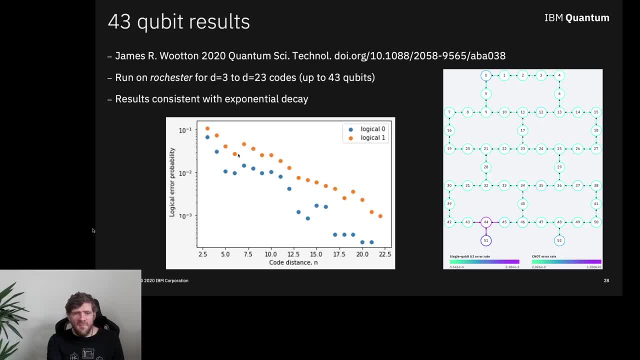 so just to show you a benchmarking experiment that I ran- and you can find this in a paper- I run it on the 53 qubit Rochester device for codes with from 3 repetitions to 23 repetitions and I looked at the probability for encoding a 0. 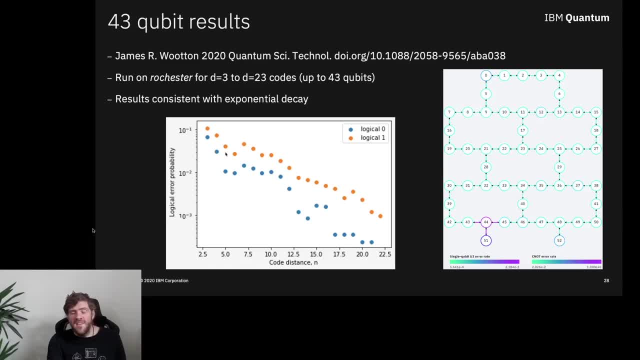 and for encoding a 1, that the decoding gives me the wrong result. and the results do show something that is a bit bumpier than theory would want, but it is consistent with the idea of an exponential decay, which is telling us that the bare minimum of what we would expect. 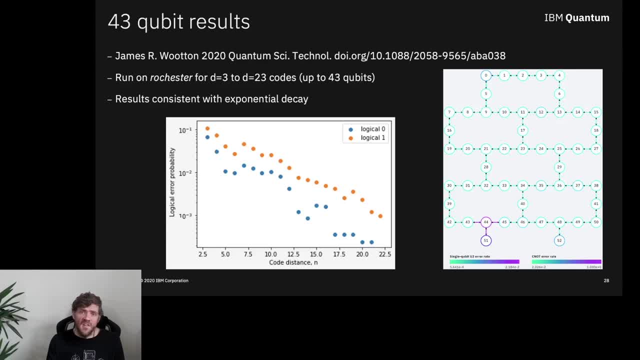 from these devices is nevertheless true, so that's pretty good. so, yeah, you can use this as like a an experiment to probe how noise is actually happening on real devices, and I've done this, of course, on a big device, using my access to such things as someone who works for IBM Quantum. 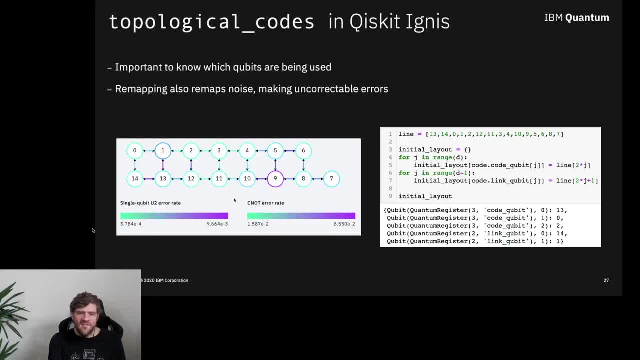 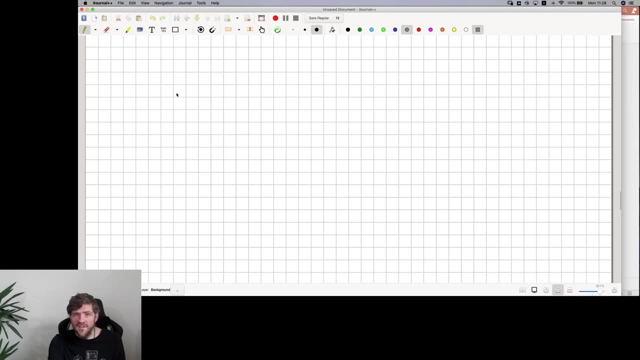 but for the smaller devices, such as this 15 qubit one, this is open for everyone, so anyone can start experimenting with noise on real devices using these methods. before we go, I can give you Shor's code, which was the one that really kickstarted quantum error creation. 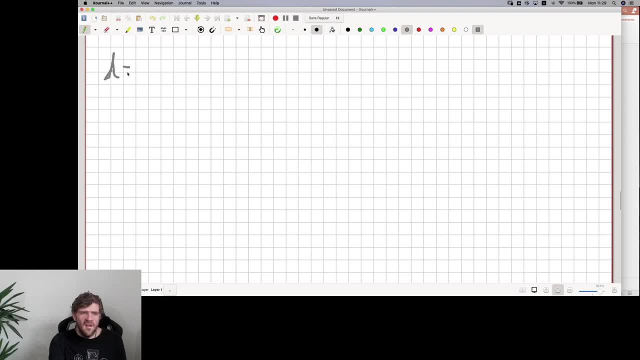 so I've talked about D equals 3 repetition codes and also I've shown you results that as you increase D up to, for example, 23 and beyond, then the effectiveness of this code increases exponentially. the probability that things go wrong decreases exponentially. it's all awesome. 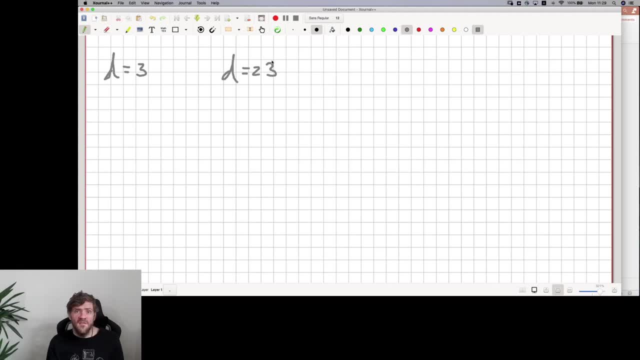 so this is one natural way to scale to get more effective repetition codes. one other way we can do it is through concatenation. so let's take 3 qubits and we effectively combine those 3 qubits in order to create one less rubbish qubit. 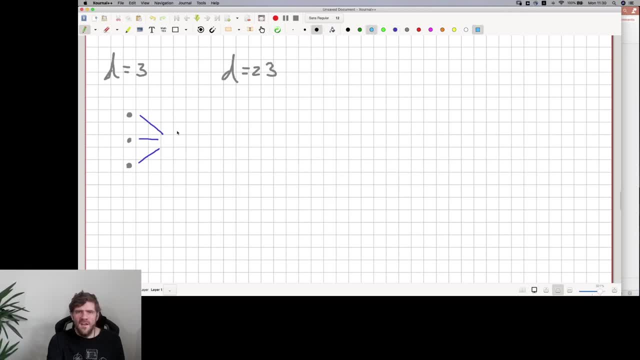 a qubit which is better protected against bitflip errors. now we want to have it even more protected against bitflip errors. so one way we could do this is to take another set of 3 qubits and combine them also with the repetition code encoding and. 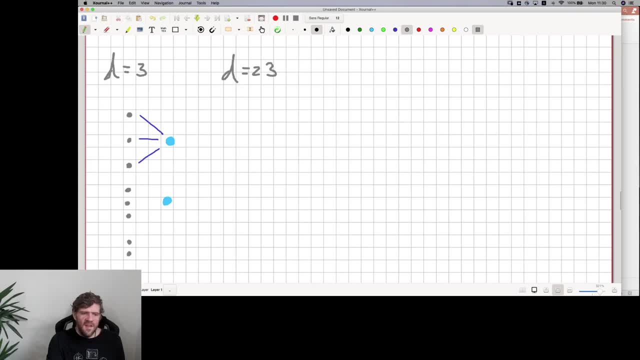 take another set of 3 qubits and combine those with the repetition code encoding and then we have 3. well, not quite physical qubits, because they've been improved a bit by encoding, but not quite logical qubits. they've only been improved a little bit. 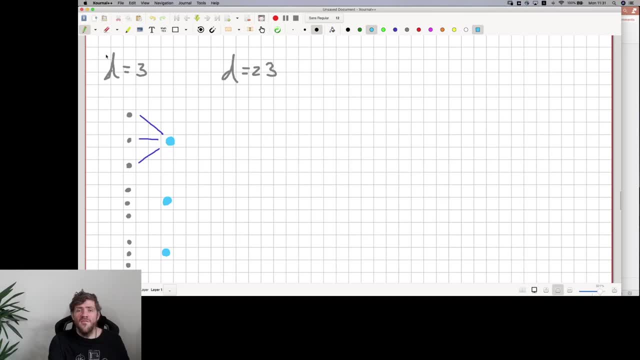 so we can then take those 3 and use those as the basis for another level of repetition code in which we combine those and we get an even more protected qubit. so this is made up of these 3 qubits, but these 3 qubits are each made up of: 3 qubits, so we've actually got 9 qubits involved here all working together to make one quite protected against bitflip's qubit, and then we can do this again, take 3 of those and concatenate them to make an even more protected qubit, and so on and so forth.